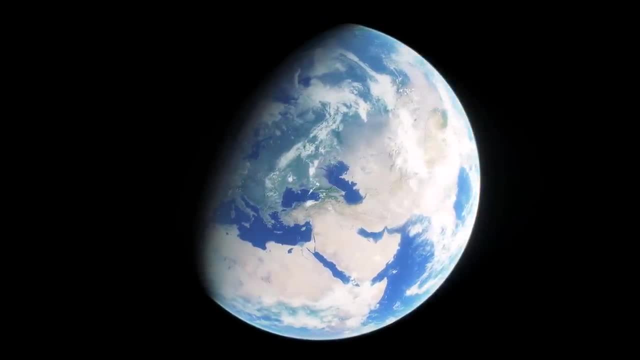 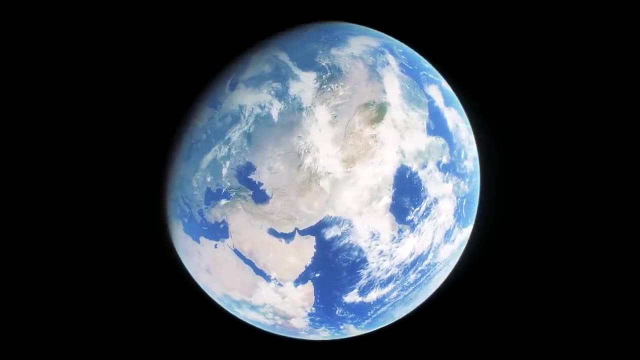 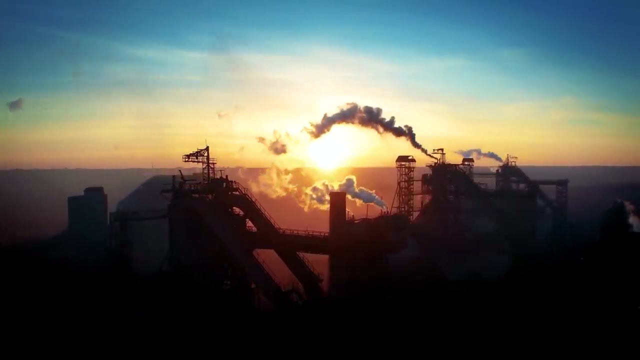 So if our goal in searching the cosmos is to discover alien life or even a second home for humanity, our best bet will be finding a planet akin to our own. And let's be honest: only a few hundred years into industrialization and we're already altering the planet in some dramatic and dangerous ways. 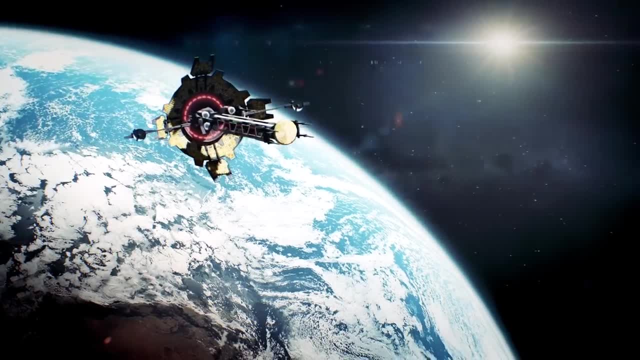 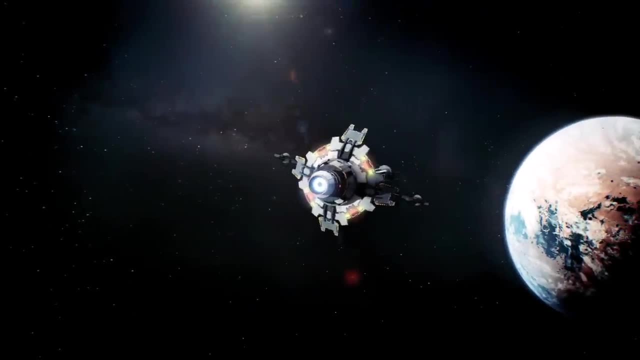 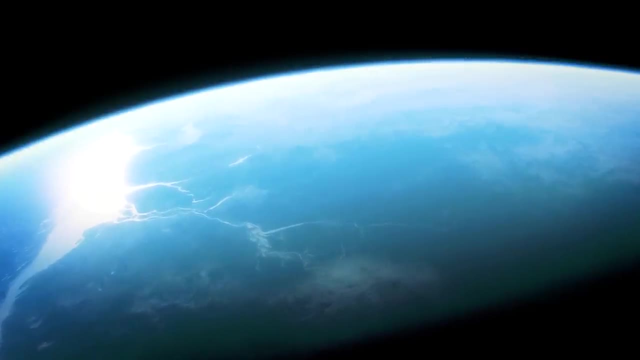 It's not entirely bizarre to think that one day, whether it's decades, centuries or millennia away, one day we will need to leave and find a new planet, preferably one similar to this one, to call home. The only problem with using ESI as a metric is that Earth-like doesn't necessarily equate to habitability. 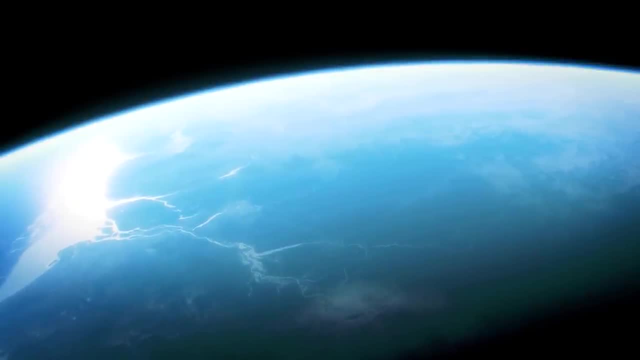 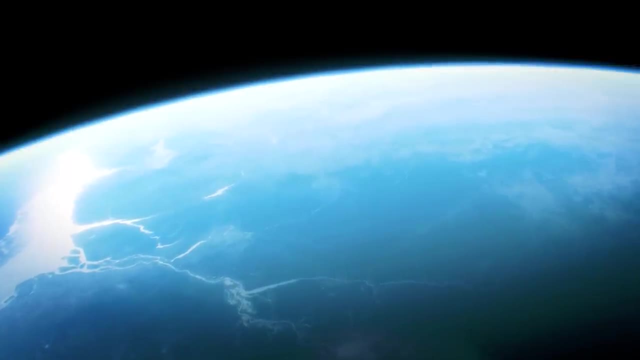 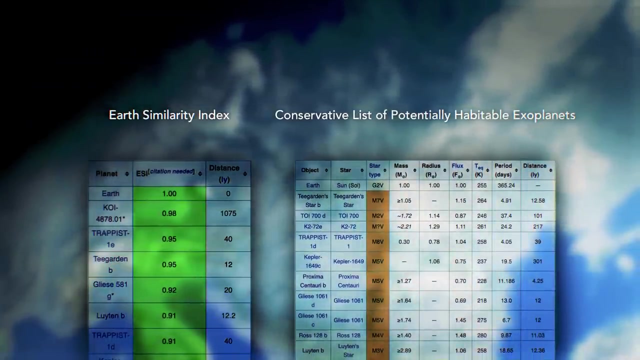 as it's possible for planets to be even more habitable than Earth, Which would simultaneously- almost paradoxically, make it less Earth-like. To mitigate this disparity between Earth-likeness and habitability, I've taken the Earth Similarity Index and cross-referenced it with the conservative list of potentially habitable exoplanets. 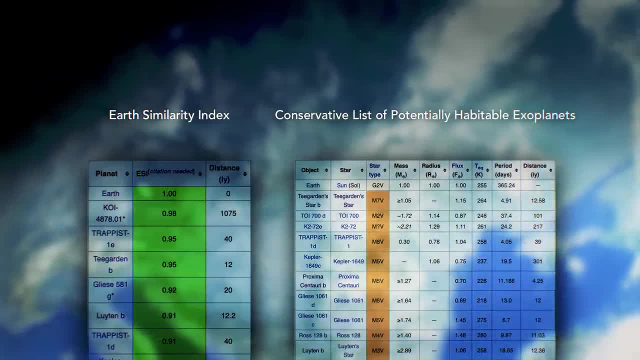 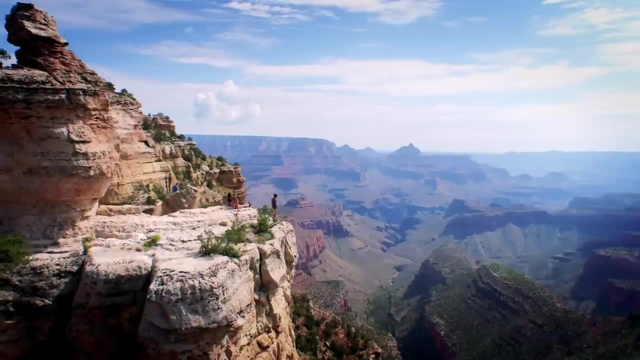 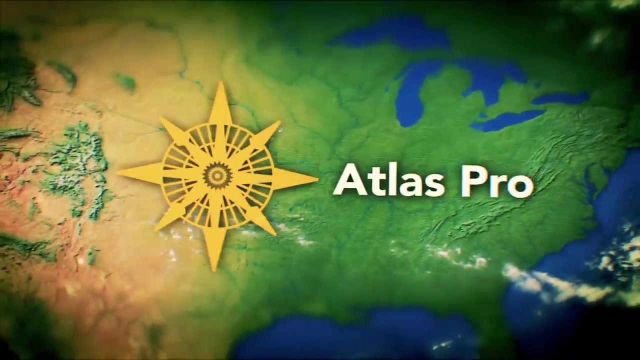 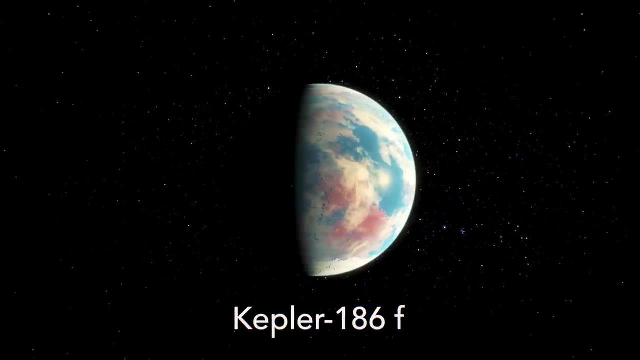 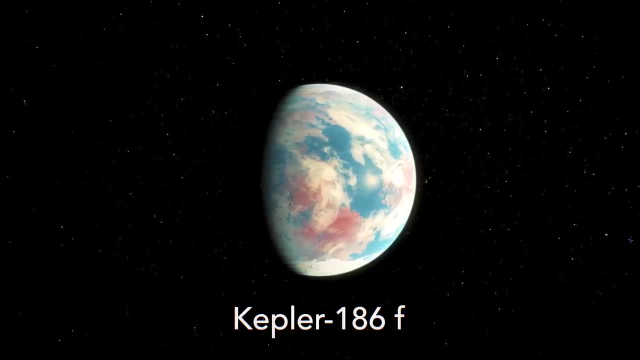 The result is a list of only the most habitable and most Earth-like planets discovered to date, or in other words, 16 candidates for Earth 2.0.. First up is Kepler-186f, With a radius measuring only 11% larger than the Earth's when it was first discovered, all the way back in 2014,. this was the first Earth-sized exoplanet to ever be discovered orbiting within its star's habitable zone. 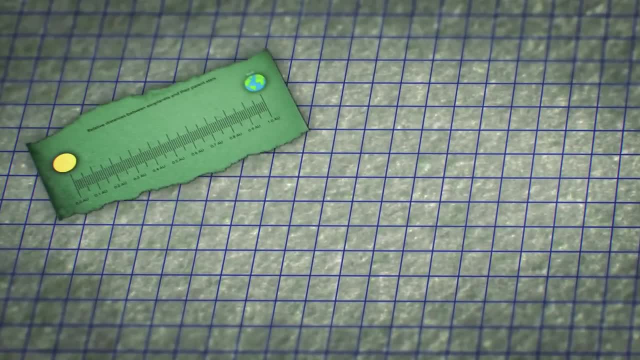 However, because the planet belongs to a much smaller and colder red dwarf star, the habitable zone occupies a much tighter area. However, because the planet belongs to a much smaller and colder red dwarf star, the habitable zone occupies a much tighter area. 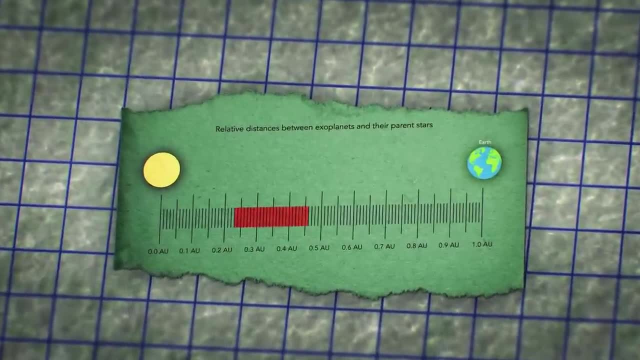 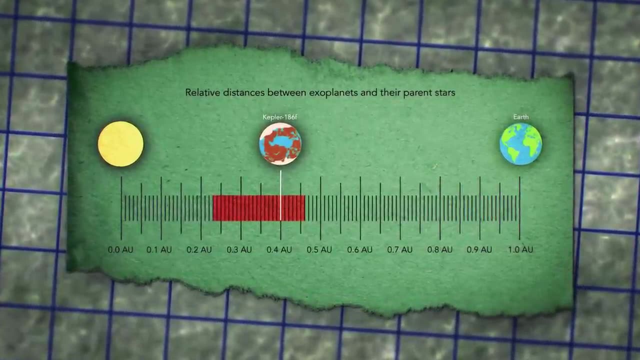 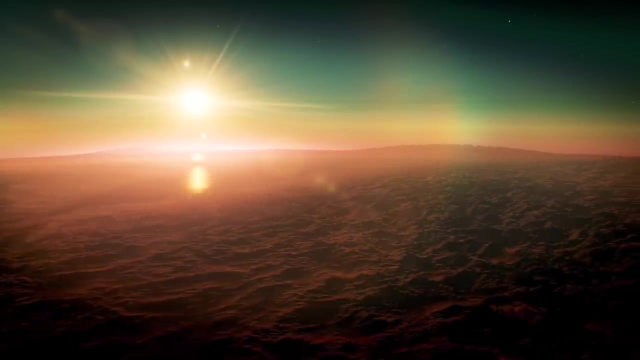 Between 0.23 and 0.46 astronomical units, Opening at 0.4 AU. this puts Kepler-186f on the cold side of its star. Despite this being roughly the same distance, Mercury orbits around the Sun. 186f still only receives 30% of the illumination compared to the Earth, making this a dim world as well. 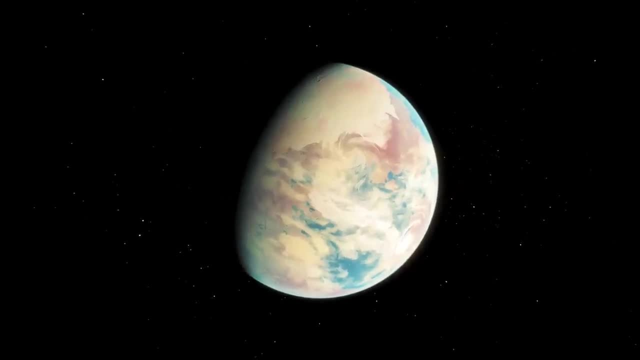 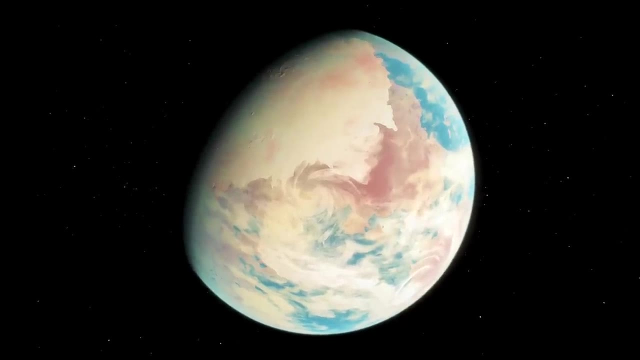 If water is in fact present on the planet in large quantities, most of it would likely be tied up in tremendous polar ice caps, Relegating the habitable portion of the planet to the equatorial regions where large lakes may be able to form. 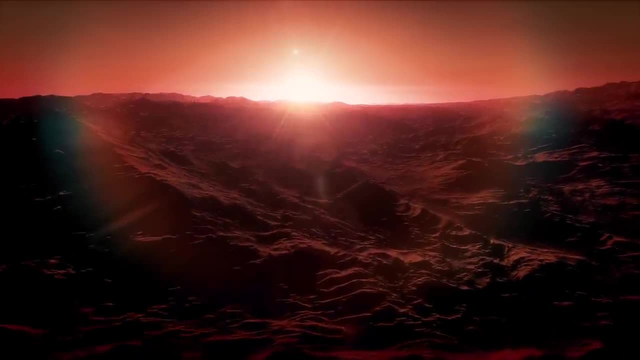 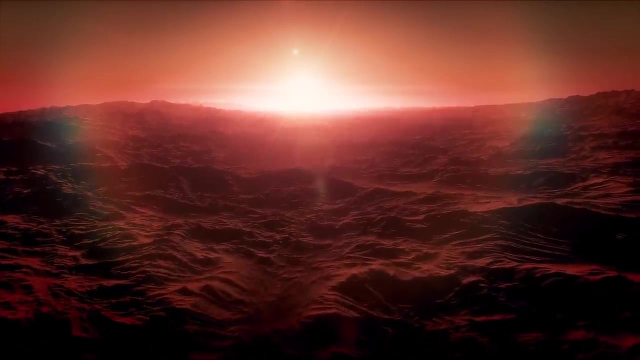 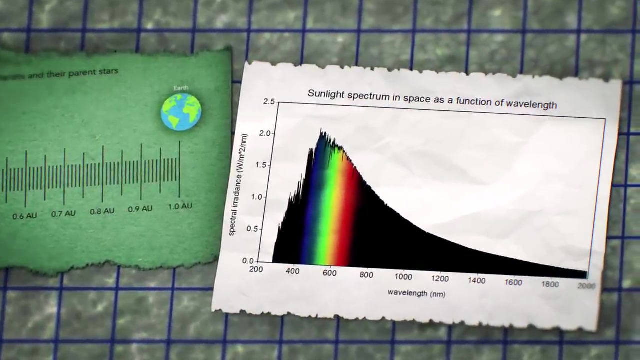 Here, life would be more than possible. but being a world bathed in the red light of a red dwarf plant, life would need to adapt. On Earth, nearly all photosynthetic life takes on a green color to reflect roughly where the Sun's light peaks, in order to avoid receiving damagingly high levels of light. 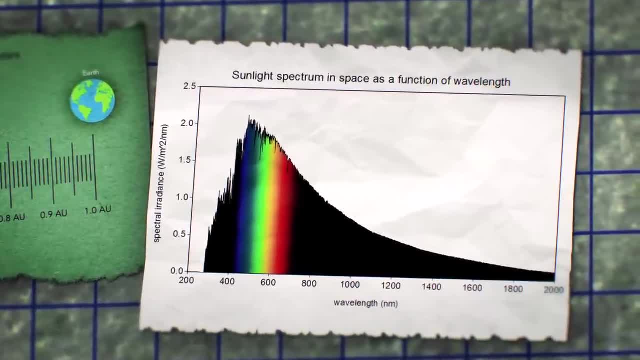 In order to avoid receiving damagingly high levels of light. Here, Kepler-186f has a more parlant color on it over the course of its entire history On Earth, nearly all photosynthetic life takes on a green color to reflect roughly where the Sun's light peaks, in order to avoid receiving damagingly high levels of light. 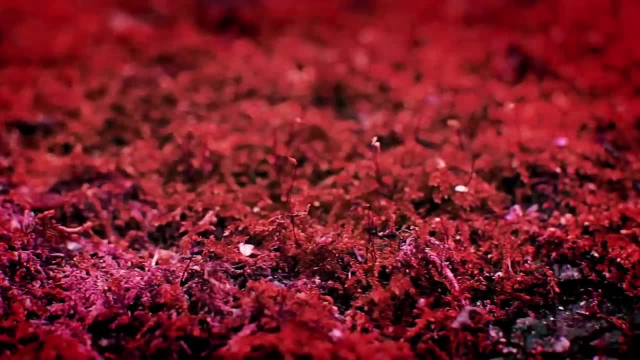 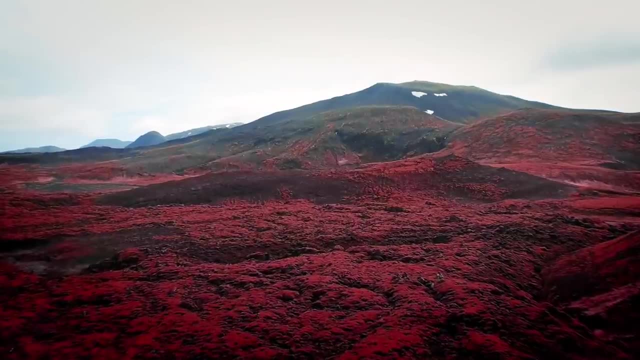 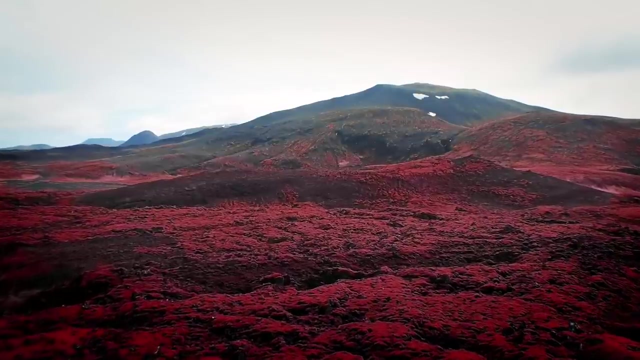 more reddish light supplied by its star, replacing green chlorophyll with a red or even purple pigment such as anthocyanin. As we'll see over the course of this video, red dwarfs serve as some of the most frequent host stars for potentially habitable exoplanets, meaning it may, in fact, be more common to find 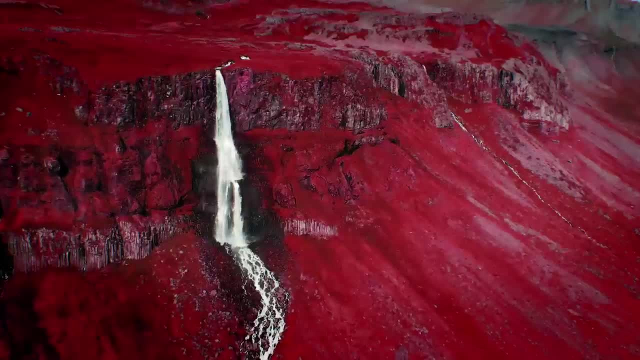 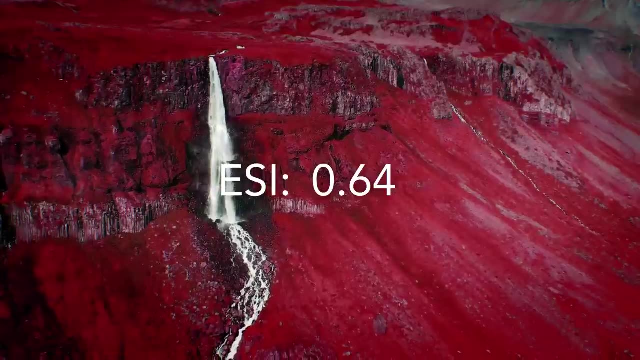 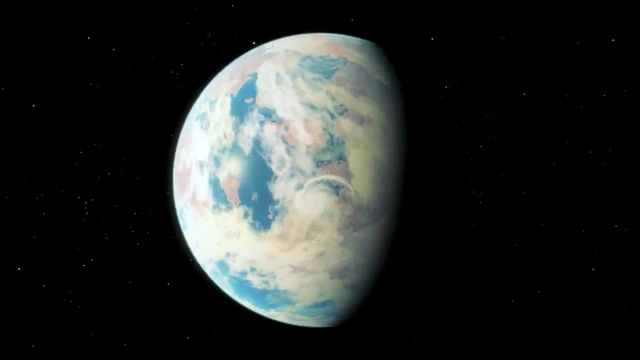 red and purple plant life than the familiar green. Overall, despite its perceived high habitability, Kepler-186f earns an ESI score of only 0.64 compared to Earth's 1.00.. That's a 64% match, which is good, but we can definitely do better. 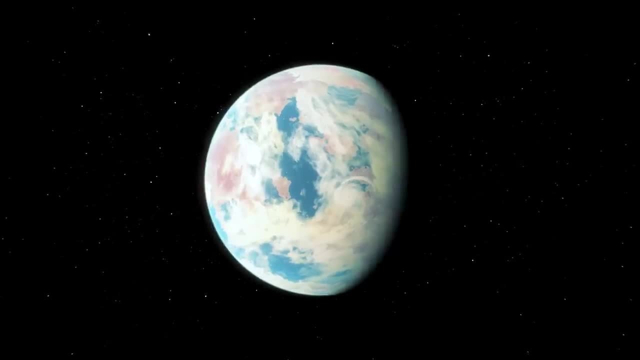 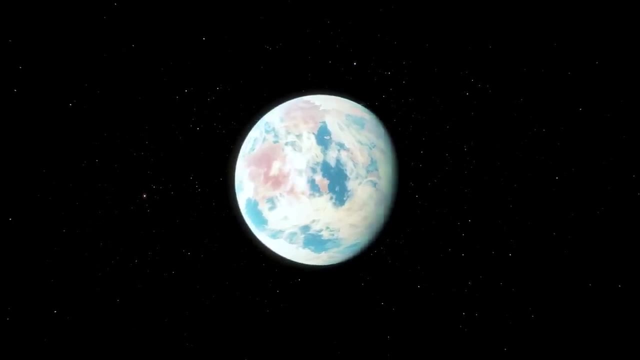 While it might be easy to wish this planet was any closer to its star, that might not be the best idea, as it's thought that 186f orbits close enough to potentially become tidally locked. Or in English, one side of the planet always faces directly towards its star and the other 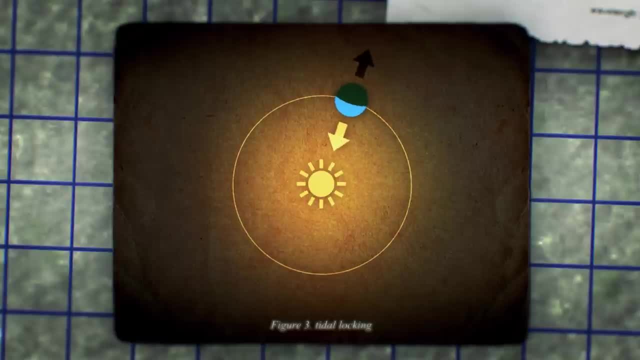 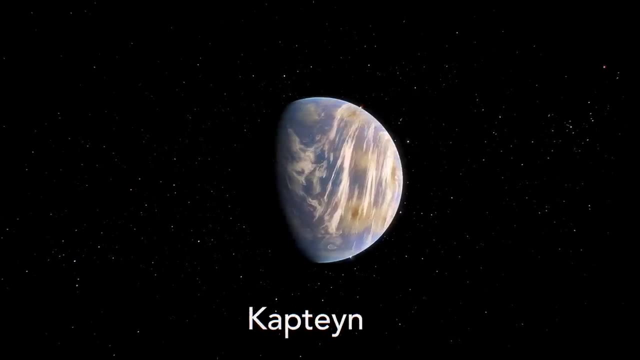 side faces permanently away. While this isn't necessarily a death sentence, it makes inhabiting a planet far more complicated than normal. This brings us to Kapteyn B Orbiting at only 0.17 AU. this gives the planet an exceedingly 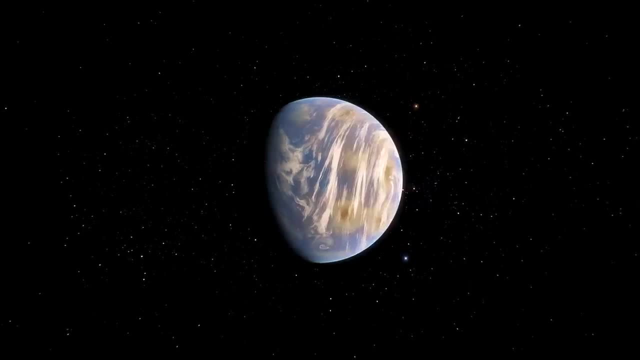 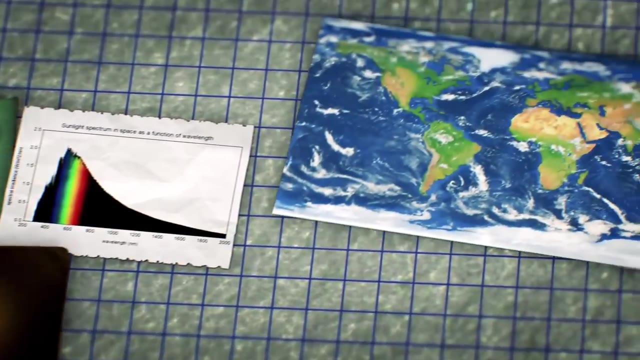 high probability of tidal locking. The biggest effect this has on the planet is how heat is distributed across its surface. On Earth, our rotation exposes all sides of the planet equally to the sun, leading the equator to receive the greatest amount of heat energy and the polar regions to receive 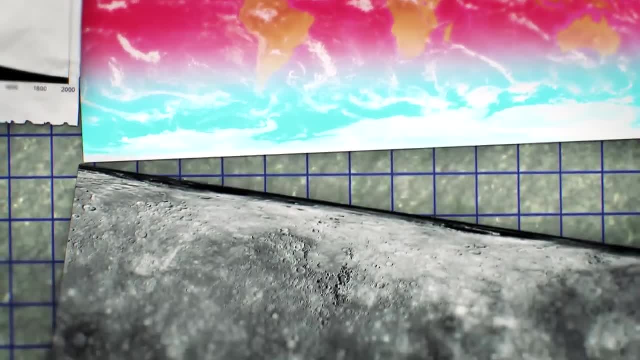 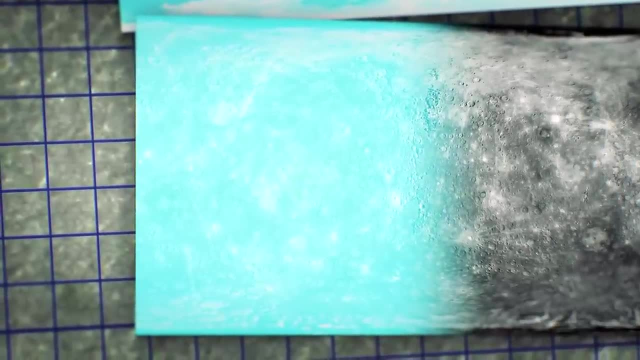 the least On a tidally locked planet like Kapteyn B. this is the highest probability of tidal locking On Kapteyn B. however, one side sits in eternal nighttime, usually resulting in a frozen wasteland where nothing besides ice crystals is capable of growing. 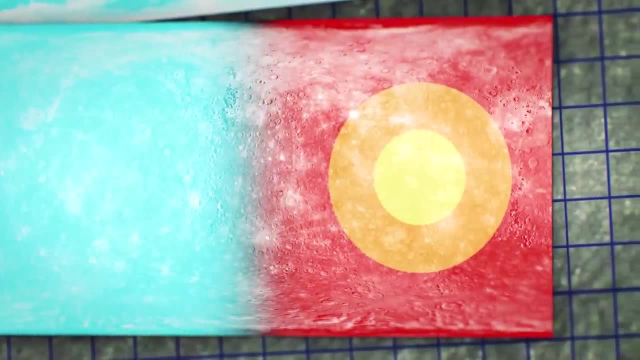 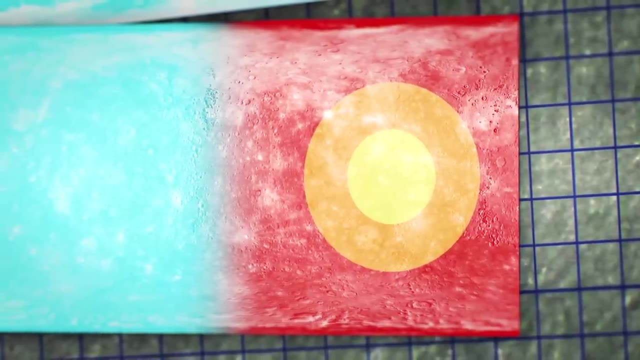 On the other side, instead of an equator, the sun's energy comes to a focus where continual daytime sends surface temperatures to scorching levels, While typically this makes the focus as uninhabitable as the other side, somewhere between the freezing. 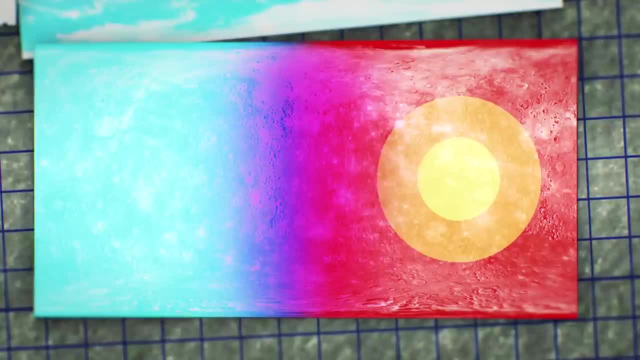 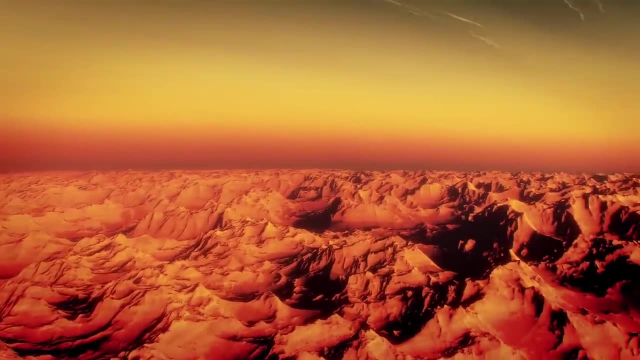 cold and scorching hot. ambient heat and partial exposure to sunlight can induce moderate temperatures and generate a narrow region of habitability. Living here, the sun would be in eternal sunset, with the skies split between a light side and a dark side. 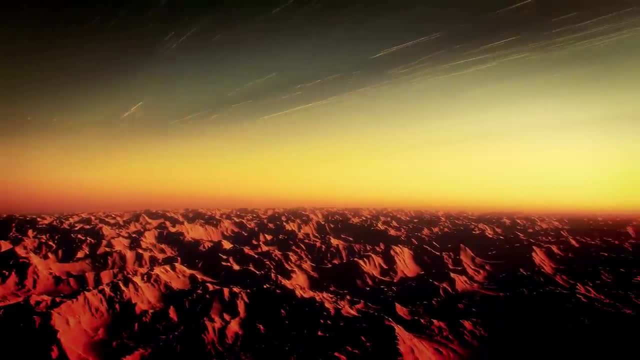 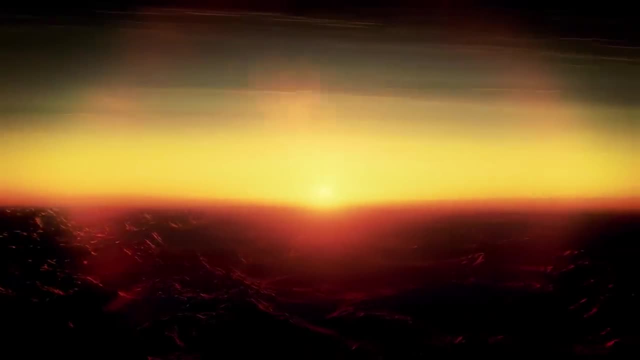 Mountain ranges in this twilight zone would be ideal for habitation, as their faces would receive light and heat up their adjacent valleys, while shielding any life from the constant onslaught of radiation. One easy way to tell if a planet is tidally locked is to look at its clouds. 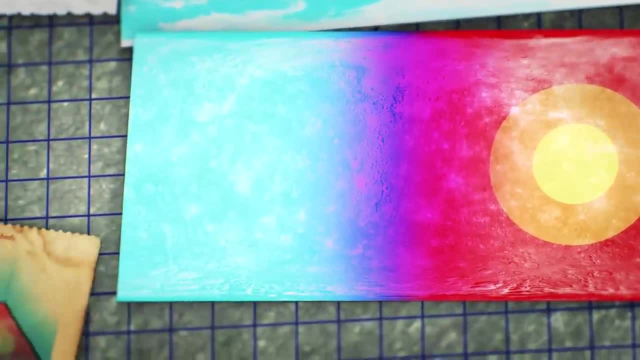 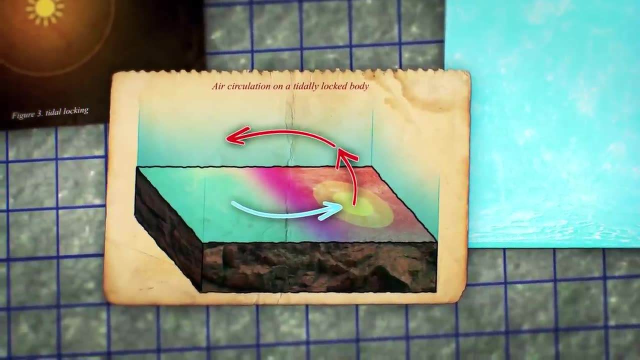 The sun is the only way to tell if a planet is tidally locked because heat is focused at a single point. Here you'd get a constant stream of warm air rising, drawing in more dense cold air from the darker side. As this warm air rises, it will cool, with any moisture condensing out into clouds, resulting. 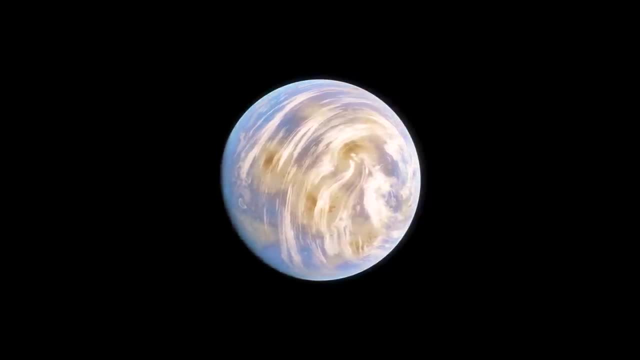 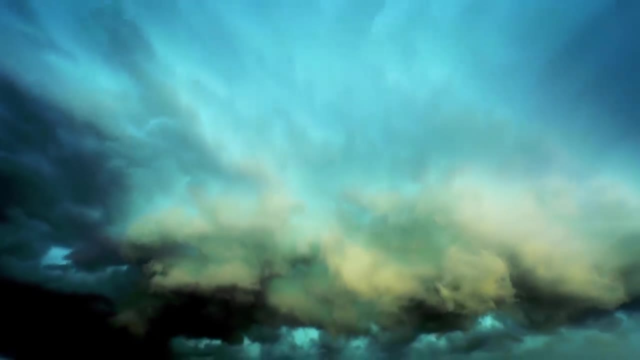 in a radial pattern emanating outwards from the focus. This one-directional air circuit would help in the distribution of heat around the planet, bringing warm air to the cold side and cold air into the warm side, helping to widen the zone of habitability on the surface. 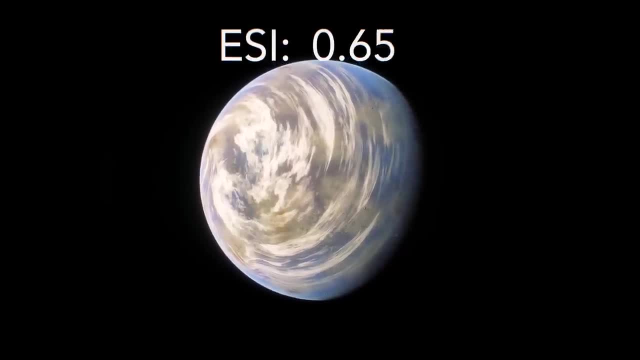 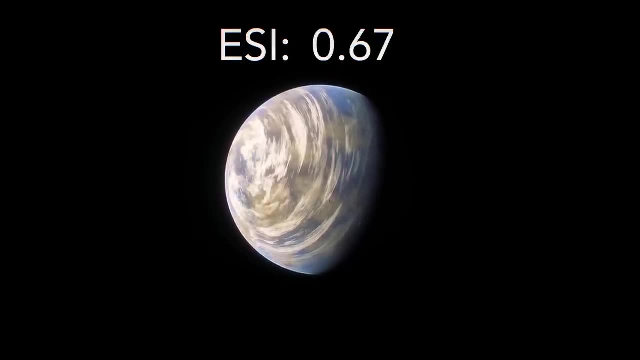 Overall, Captine B earns an ESI of 3.5.. And the ESI of the Earth is a high ESI, with the ESI being the highest of the best. Captine B earns an ESI of 0.67, which admittedly still isn't very high. 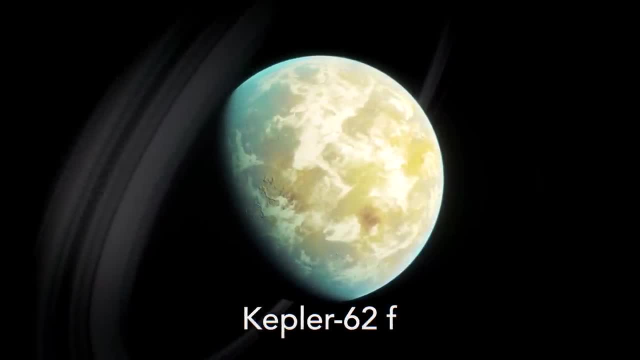 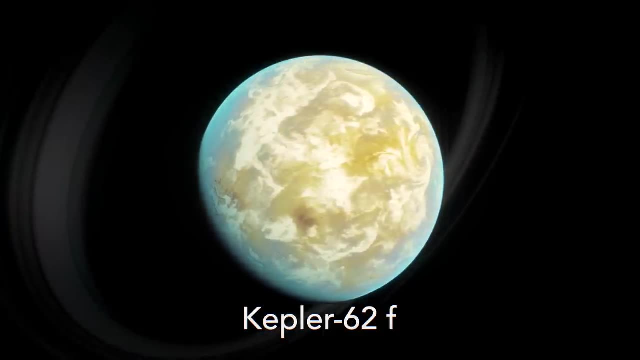 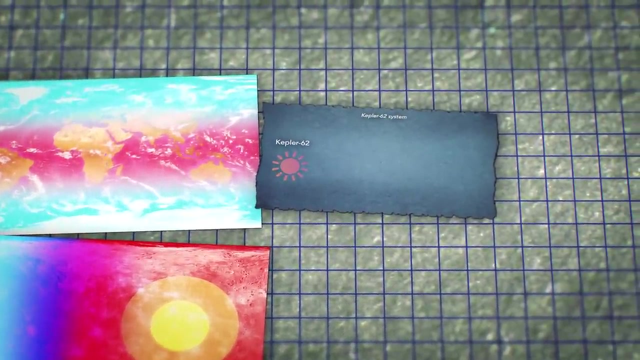 Making up for this is the fact that Captine is only 12.8 light years away, making a visit here slightly more possible than, for instance, Kepler-62-f, which orbits a star some 1,200 light years away. If you've been wondering how the names of these planets work, Kepler-62 refers to the 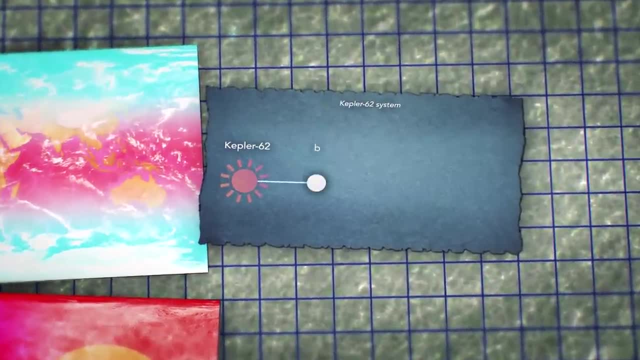 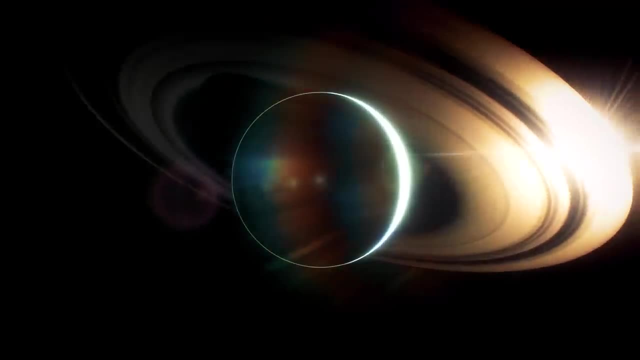 central star with F means that there's a coupler- 62B, 62C, 62D and 62E- before getting to 62F. With so many planets packed in, it's no surprise that 62F is relegated to the far. 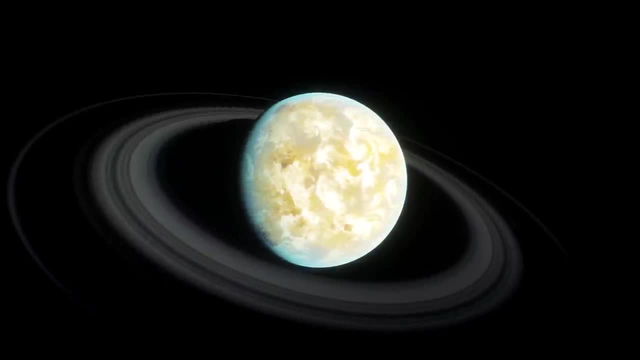 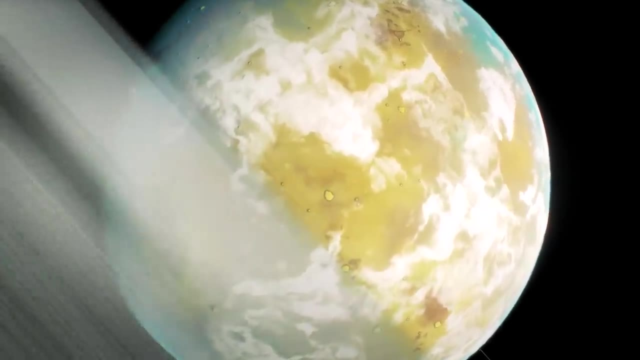 side of the star's habitable zone, making it another cold world. This might not be such a bad thing, however, given how big the planet is, at over 1.4 Earth radii. At this size, the planet would be much more likely to have a molten metal core. the benefits: 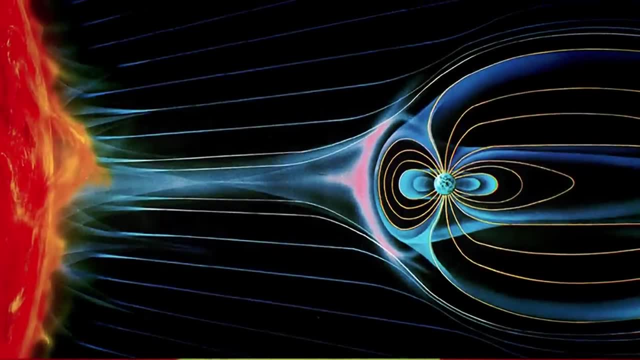 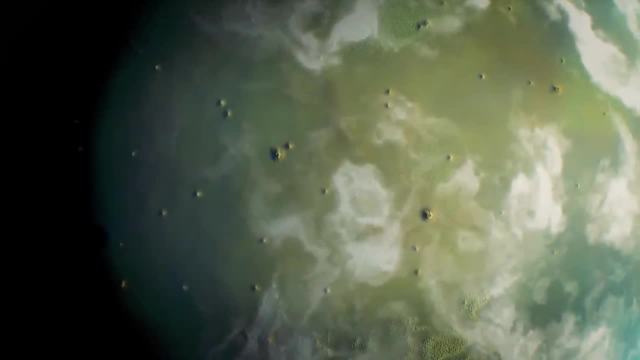 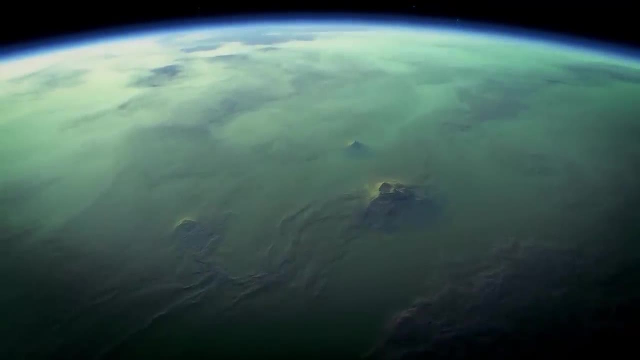 of which not only being the capacity to propagate a strong magnetosphere capable of protecting the surface from potentially damaging radiation, but also powering robust geologic activity, helping the planet to build an atmosphere through volcanic outgassing and generate a greenhouse effect. to hold on to what slight amount of heat energy comes the planet's? 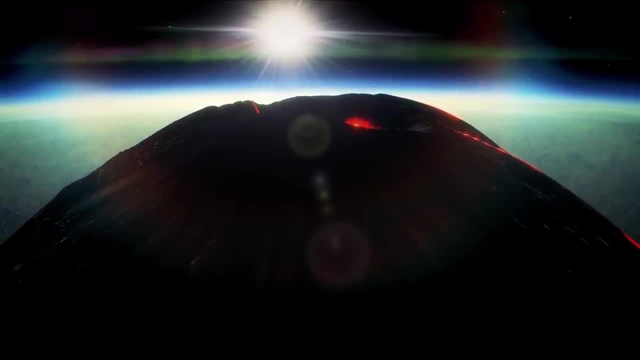 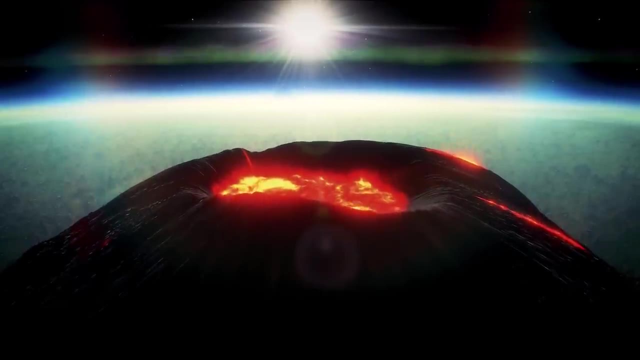 way. Ultimately, Kepler-62F's habitability all boils down to how thick of an atmosphere it has, with calculations showing that at least five Earth atmospheres of carbon-dioxide would be needed to sufficiently trap enough heat to melt ice on its surface. 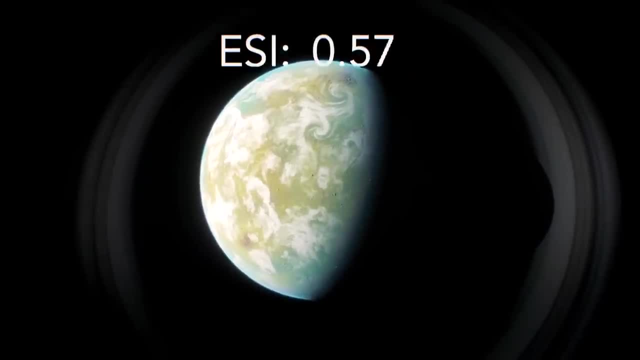 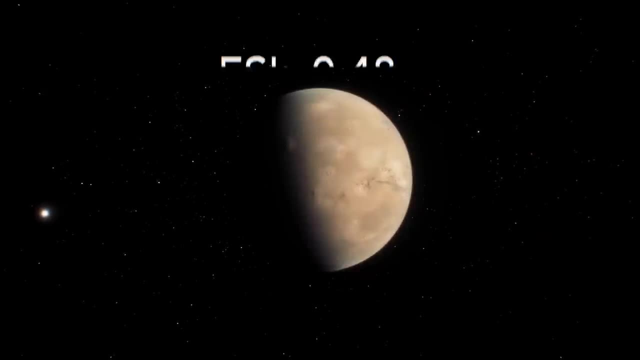 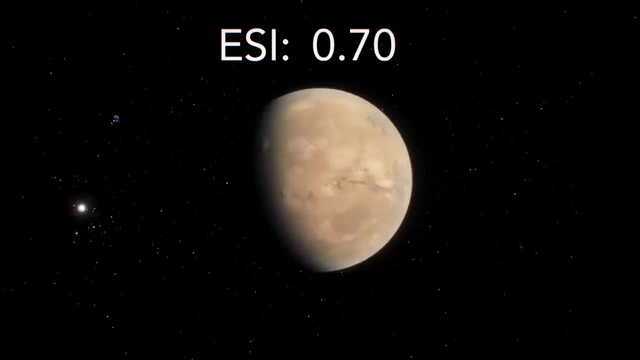 All of this considered, Kepler-62F earns an ESI of 0.69, and it's at this point that we've reached an important distinction in our rankings, as Mars has an ESI of 0.70.. This gives us not one, but two points of reference, and places all the upcoming planets somewhere. between these. Given that we believe Mars could have supported biologic activity earlier in its life, this means the planets that fall within this range all have a very good chance of being able to do the same. This brings us to Kepler-22B. 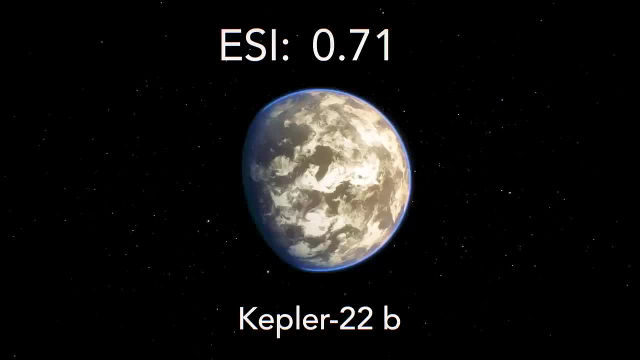 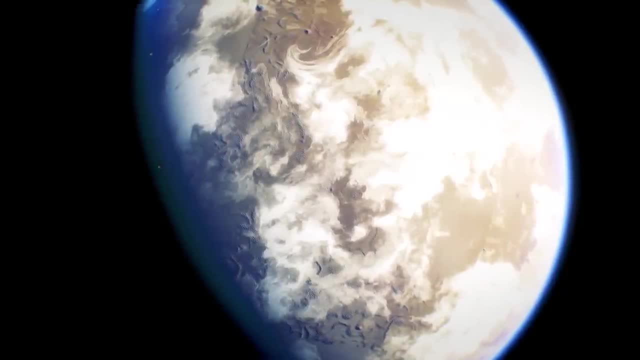 With an ESI of 0.71, here we'll find a planet that is only marginally more Earth-like than Mars, At over 2.4 times the size of the Earth. this starts getting into territory of what we'd call a super-Earth. 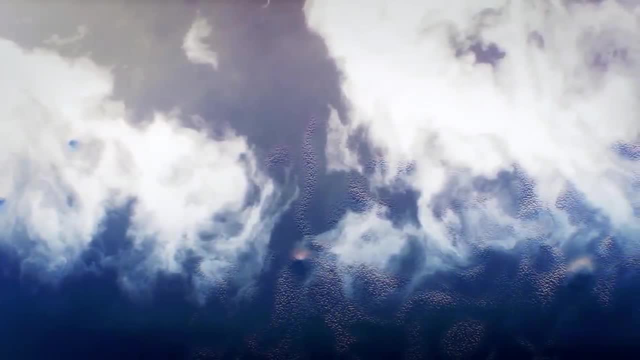 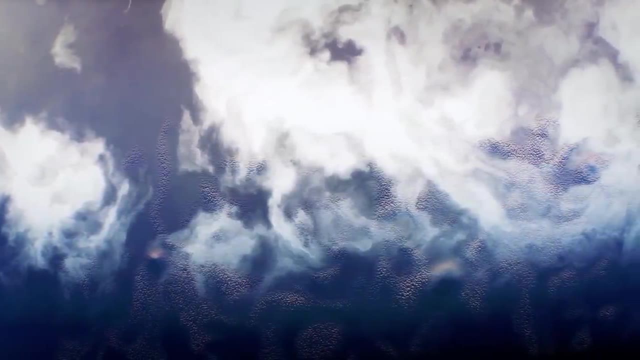 Based on computer models. if Kepler-22B features an atmosphere of similar composition to the Earth's average, surface temperatures here would reach around 20 degrees Celsius. It's only slightly warmer than the Earth's average of 15 degrees Celsius and very nearly 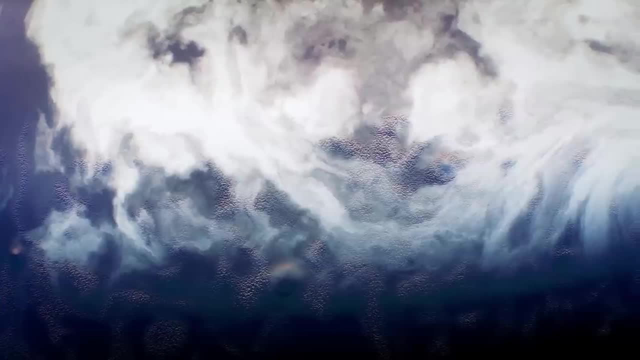 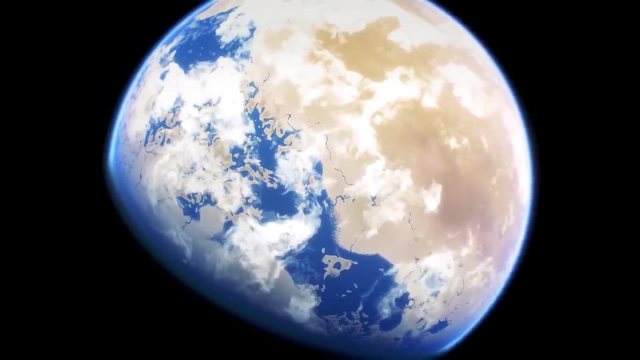 equal to the average 20 degrees Celsius experienced by Earth during its early Carboniferous period. Not only does this place 22B comfortably within the habitable zone, but also means liquid water on the planet's surface is not just possible, but rather probable. 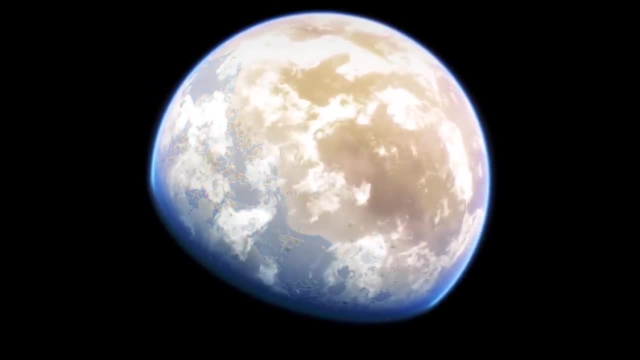 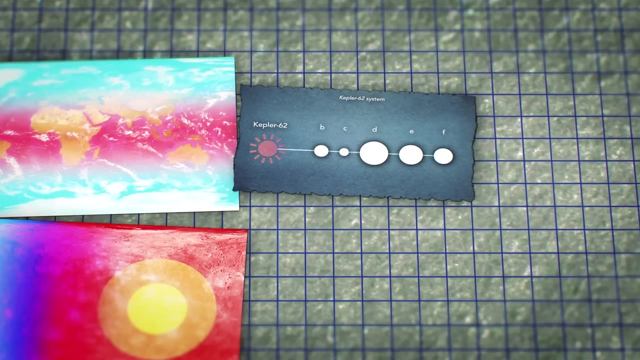 However, warm temperatures are only one of two conditions necessary for liquid water to exist on the planet, The other being, well, the presence of water, which isn't always a given. You see, the amount of water a planet has is often determined early in its creation. 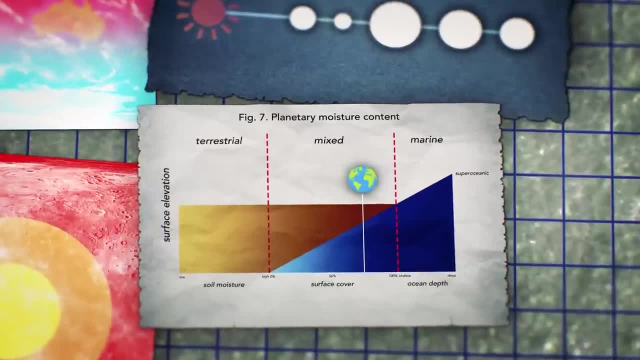 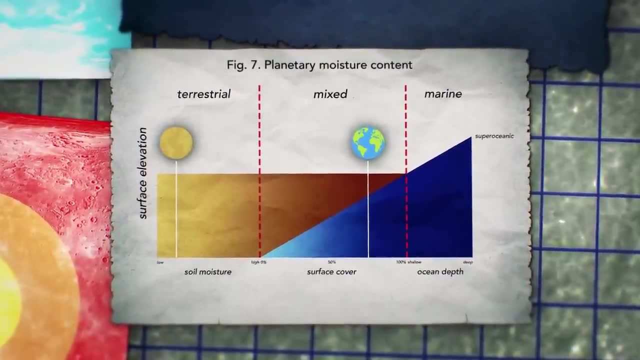 If a planet is lucky, it could end up like Earth and receive an intermediate amount of water, leading to the creation of both marine and terrestrial environments. But if far less water was available in the early days of planetary formation, an entirely terrestrial environment could result. 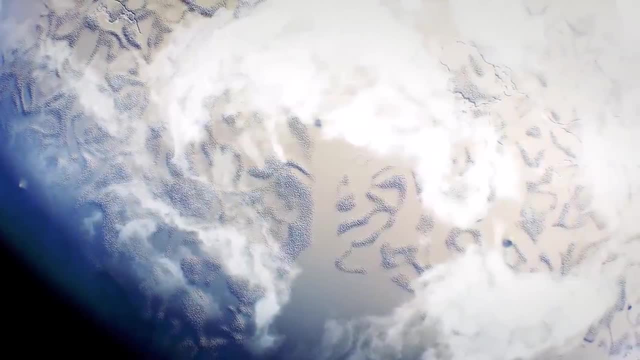 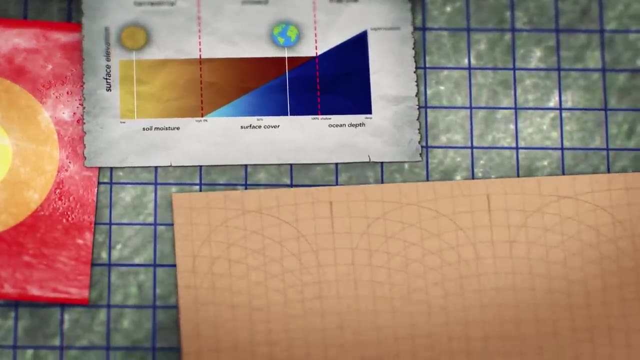 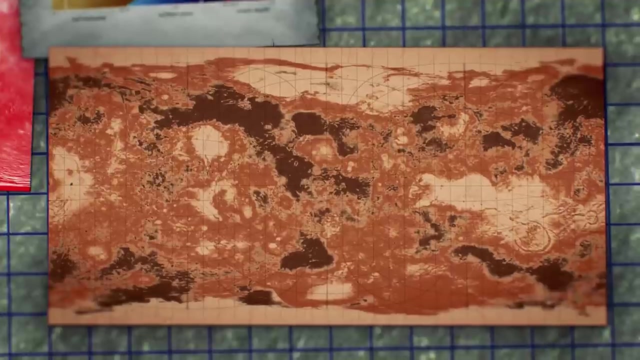 Without enough water to form stable liquid bodies, the greatest concentrations of moisture on the planet would be found within the soil. A proper map of a world like this would replace oceans with vast pools of mud, swapping out continents for extensive areas of routinely dry ground and, in the place, of large ice. 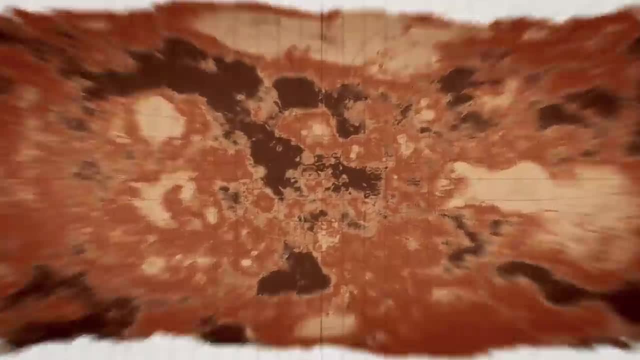 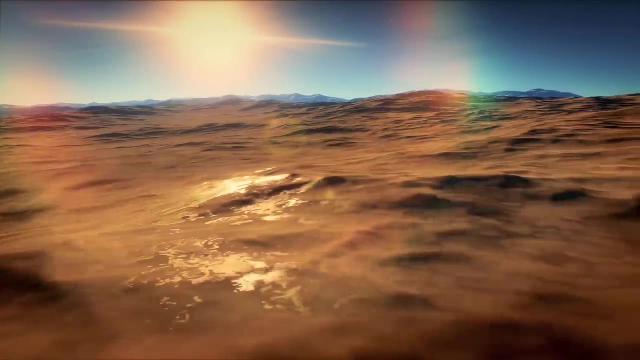 caps would be lands of thorough permafrost. While these conditions might be less than ideal for the development of life, if you know your soil science, then you'll be aware that moist dirt is one of the best environments for microbial life to thrive in and here on Earth, it is within the soil that life 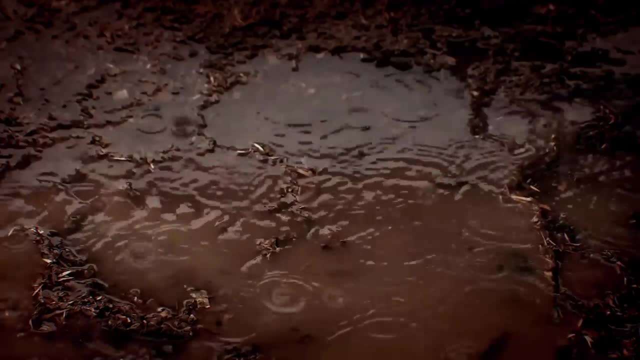 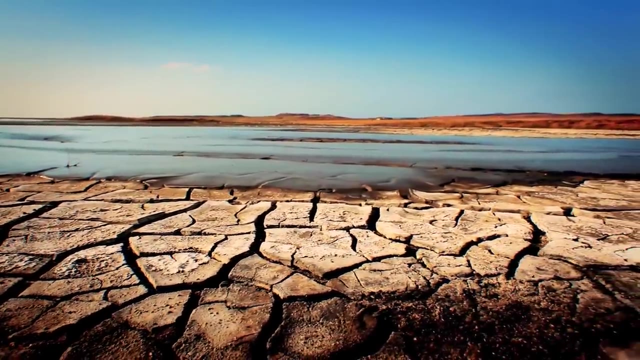 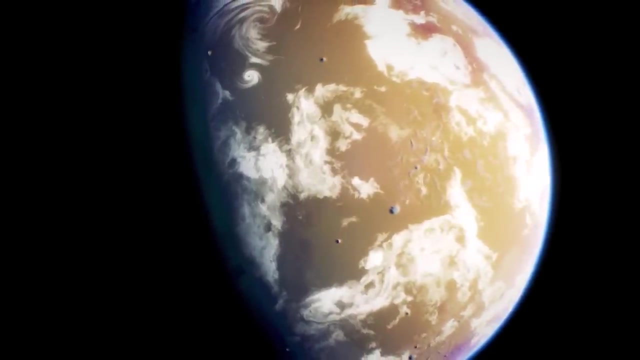 becomes more abundant and diverse than any other ecosystem on the planet. Much the same would be expected of an arid world, where any potential life could prosper within the mud regions while avoiding the dry desert areas and frozen poles. Here, in the living mud pits, microbial life could even flourish to the point of altering. 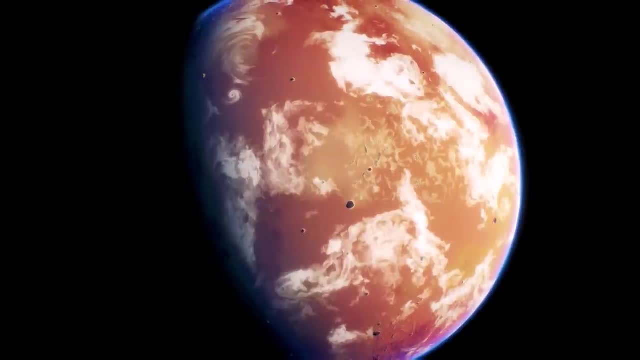 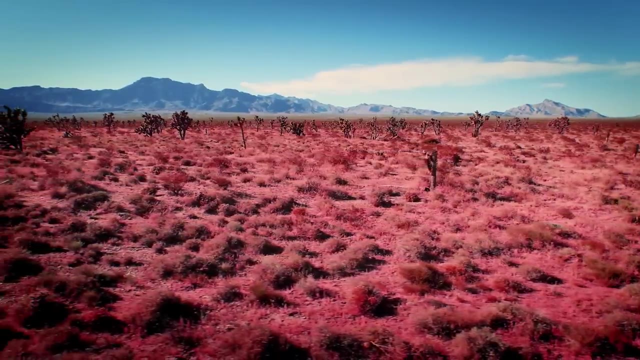 the color of the surface revealing where blooms of biological activity are taking place within Plant life isn't necessarily out of the question here either, though it's unlikely something as dense and water-consuming as forests would be able to grow and surface vegetation would. 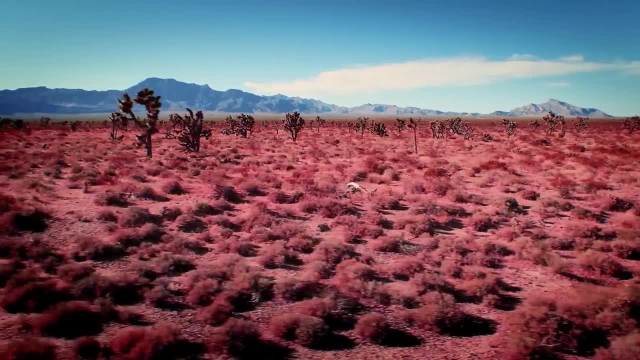 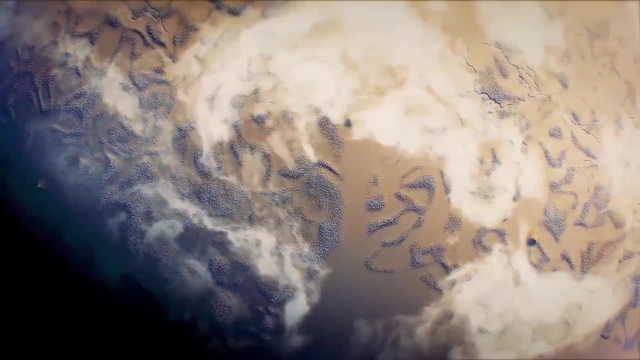 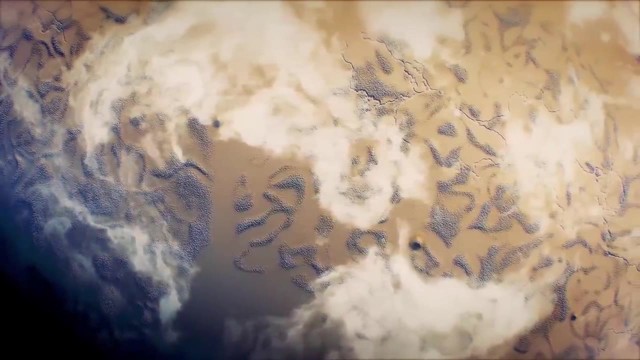 more likely consist of moss layers and maybe some sporadic standing plants. Overall, it's likely that desert planets and, by extension, living mud planets are far more common than planets like our own Earth, and future space exploration might look less like meeting a bunch of cool smart aliens and be more about logging all the 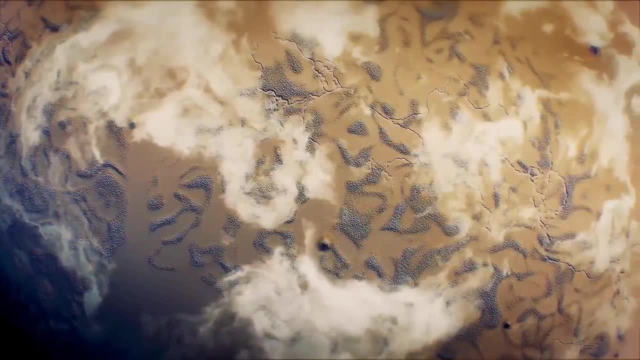 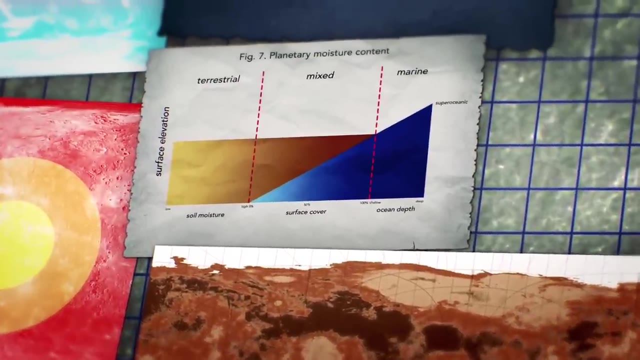 millions of different forms of microbial alien life and choosing the best ones to farm. But as our exploration of the earth is becoming increasingly complex, we'll be able to explore more of these planets in the near future. In the near future, we'll likely find that a wide spectrum of planetary moisture contents 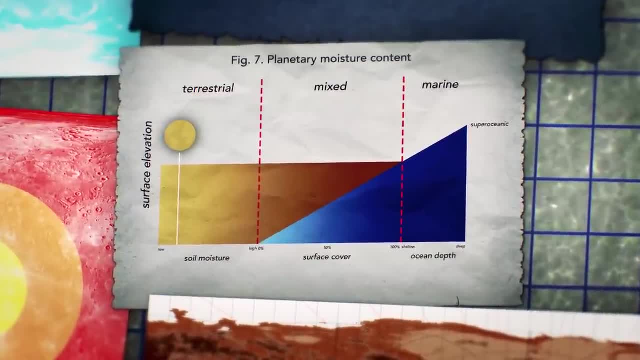 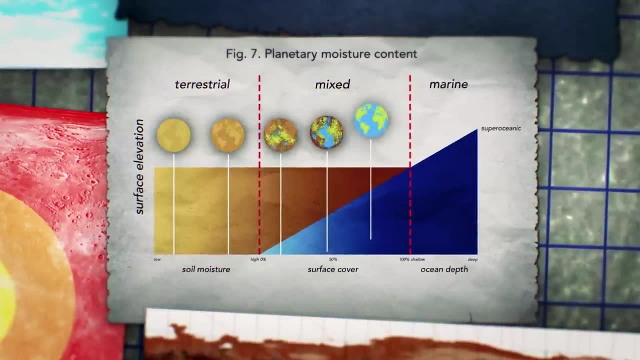 exists, ranging from a planet with only a few meager and seasonal mud collections to more established wet spots, eventually to the point where small pools are able to form, then lakes all the way to oceans, However, with hydrogen and oxygen being the most abundant and third most abundant elements. in the universe. water is by no means a rare substance. cosmically speaking, This means that, as likely as it is for a planet to receive far less water, it's likely that it's going to be more than that. In fact, in all likelihood, both fully desert planets and fully ocean planets are more common. 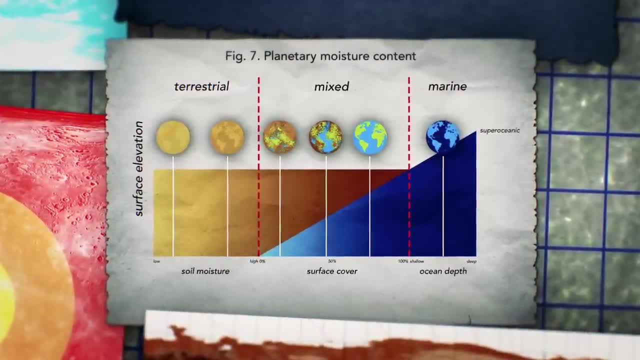 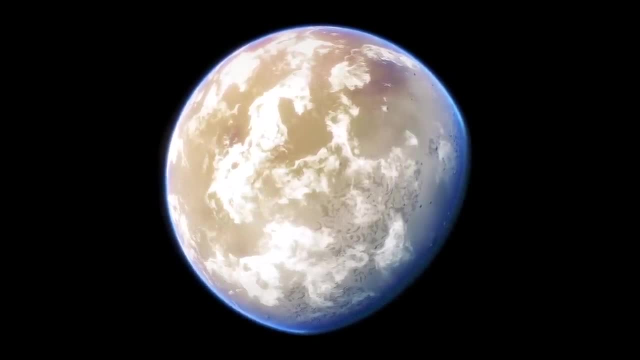 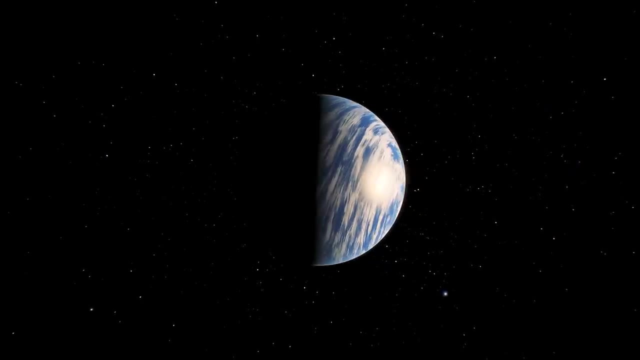 than Earth-like mixes, which require a precise balance between the two. Where Kepler-22b falls on this spectrum is unknown, though based on its size and mass, some suspect the planet could actually fall further onto the ocean side of things. For a true example of an ocean world, we can move over to our next planet. 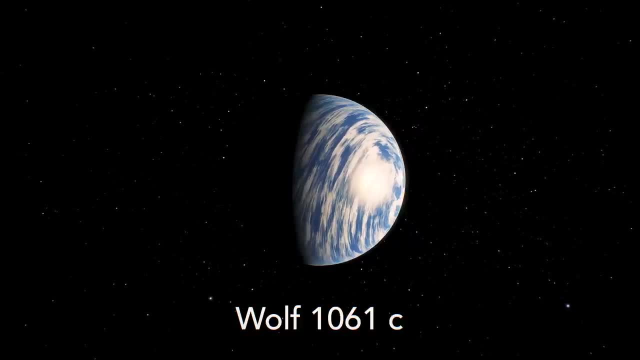 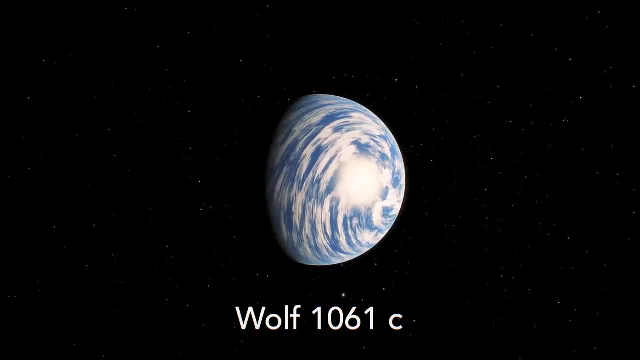 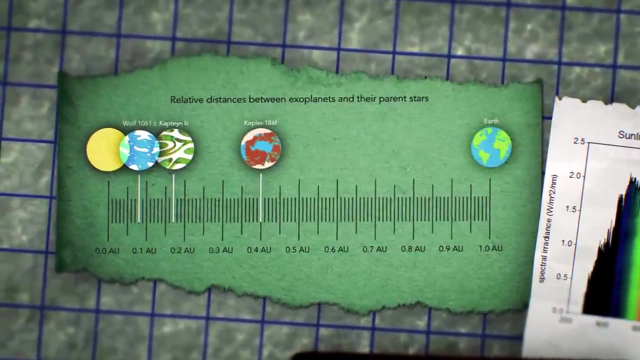 Wolf 1061c, which has been modeled here. as such, though, I should make it clear that without further study we can't say for sure what the atmospheric surface or oceanic conditions of any of these planets truly are. Orbiting extremely close to its parent star at 0.084 AU, this is almost certainly another. 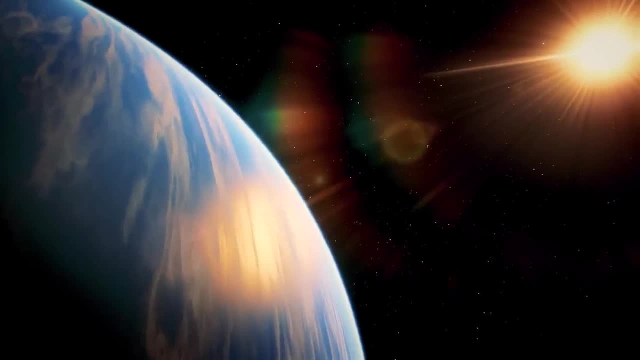 tidally locked planet, though with a luminosity of less than 1% that of the sun. this puts 1061c just within the inner edge of habitability. Now, even though this planet is a planet with a very low tidal density, it's still a planet. 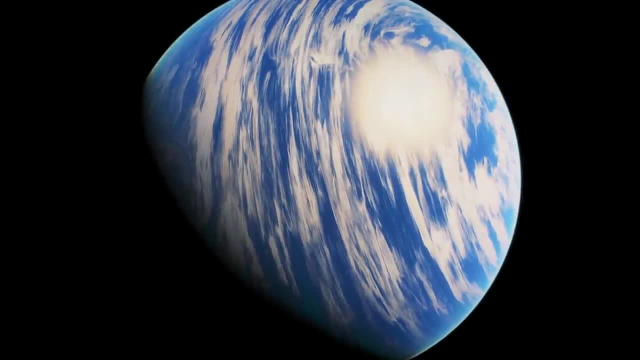 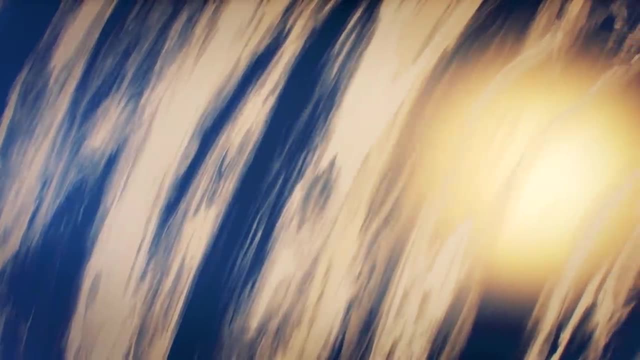 with a very low tidal density, Even though we've looked at a tidally locked planet already. the addition of a superocean reaching many miles deep at its shallowest gives us more to talk about. For starters, water is a much better regulator of temperature than air, and so warmth would 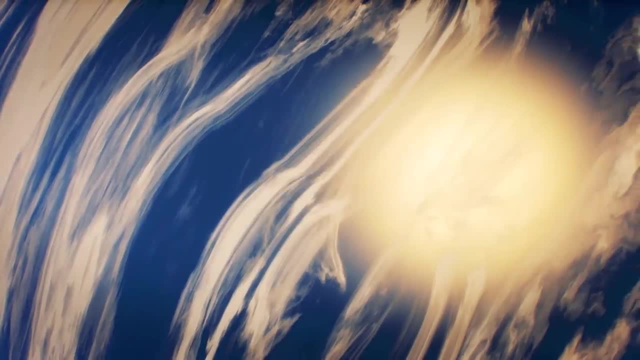 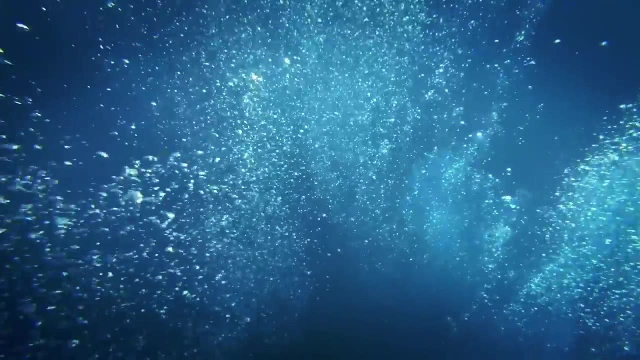 likely be far more evenly diffused across the planet compared to a solely terrestrial body, While temperatures at the focus may still prove far too hot for life and even create a zone of spontaneously boiling waters. like other tidally locked planets, there would 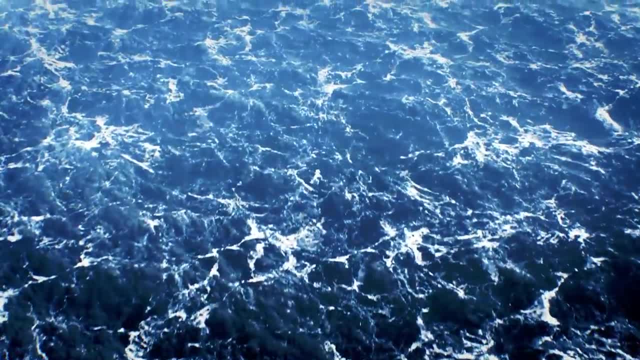 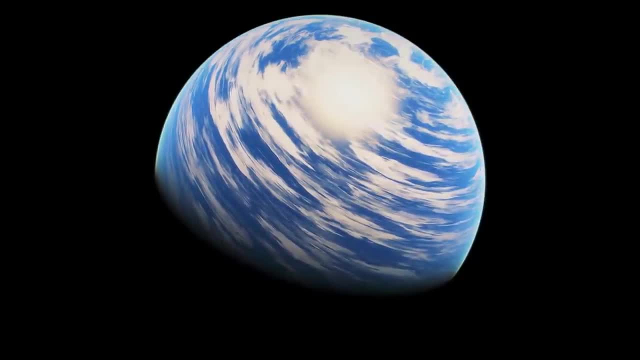 assuredly be a range of temperatures that are far too hot for life. In other words, there would likely be a ring somewhere between the hot and cold extremes where life could potentially inhabit. If Earth's oceans are any indication, so long as the water isn't frozen, it can support. 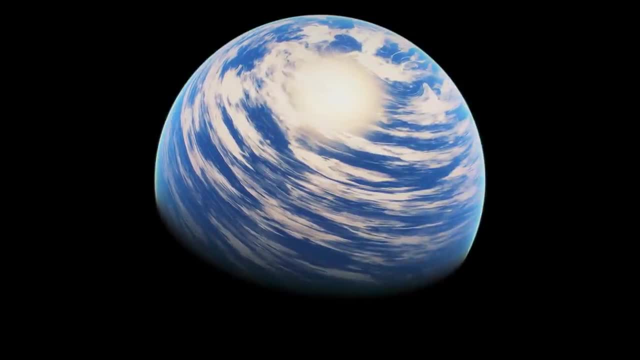 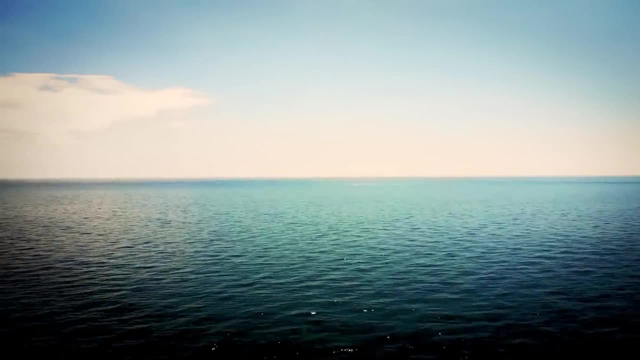 life, meaning marine life, could likely even survive on the night side of the planet, so long as the water hasn't turned to ice. Besides this, however, there'd likely be another line of potential habitability, not one at any specific longitude, but rather one at a specific depth. 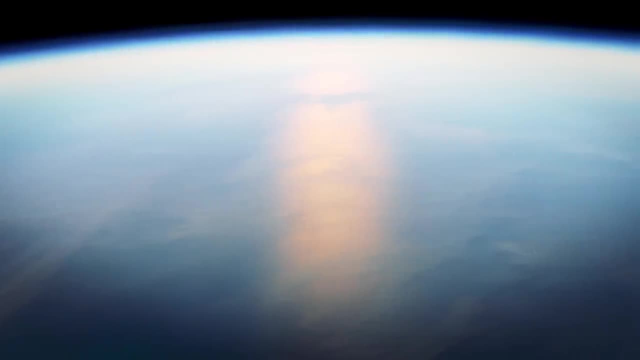 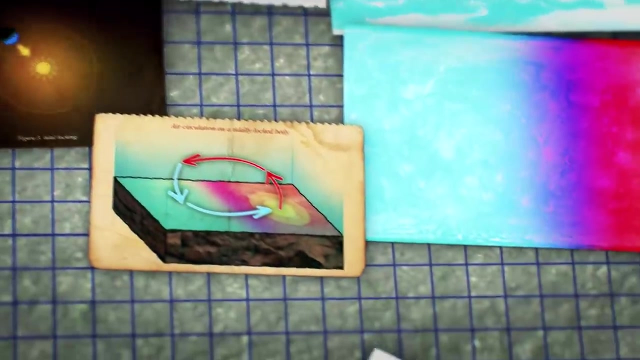 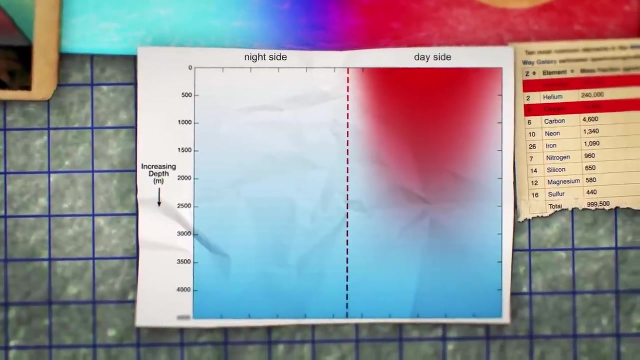 You see, on a superoceanic world like this, no matter how direct the ocean is, there's always a chance that the water will eventually cool down. This would lead to another temperature gradient deepest, directly below the focus, and trend closer and closer to the surface the further away it gets, until finally it joins the surface. 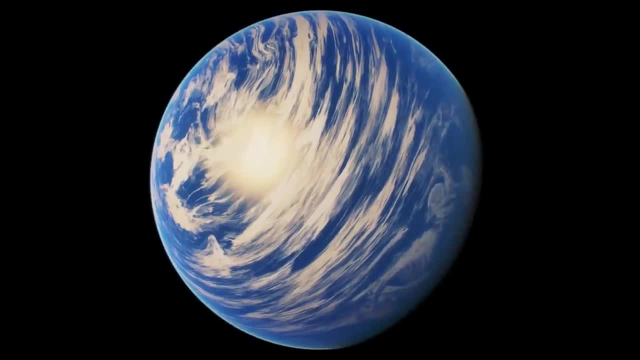 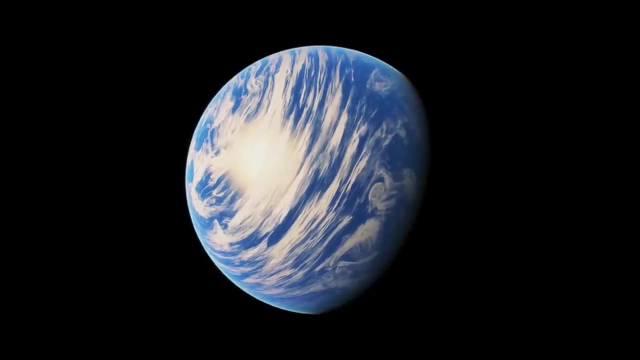 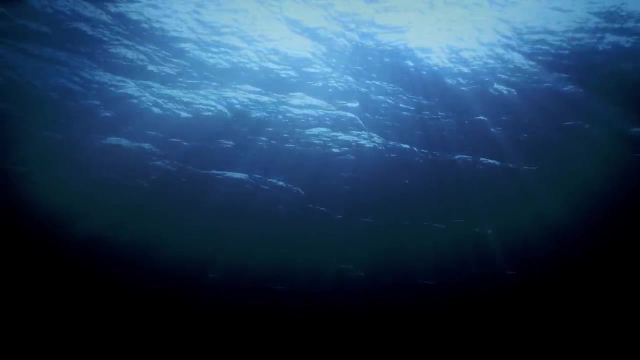 level habitable ring. What this means is, contrary to tidally locked terrestrial worlds, a far larger portion of ocean worlds would be conducive for life, and we could expect to find a tremendous diversity of biology in a place like this. A major challenge for life on a superoceanic world is that, with oceans miles deep everywhere, there'd be no surfaces for plants to cling to while still receiving light. The name of the game here would therefore be buoyancy, where nearly all life would be responsible for keeping itself afloat indefinitely. Photosynthetic life could come to rely on pneumatocyst-type structures to keep afloat. like kelp does. here on Earth, Animals would either need to employ swim bladders or carefully balance their body structures to remain neutrally buoyant. But, honestly, there are so many tactics organisms could employ to survive in a place like this that it's almost impossible to pinpoint what exact evolutionary paths might be taken. 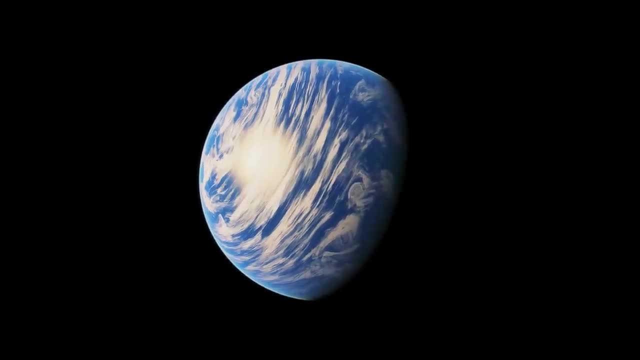 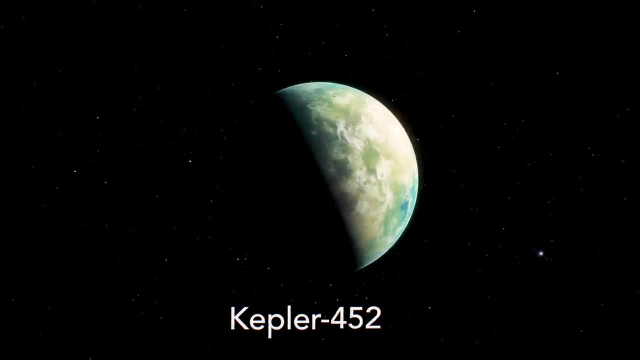 here. Overall, the potential for life to exist on a planet like this supports Wolf 1061c scoring an ESI of 0.76.. Next up we have Kepler-452b At 1.5 Earth radii. this would be another super-Earth and gets bonus points for orbiting. 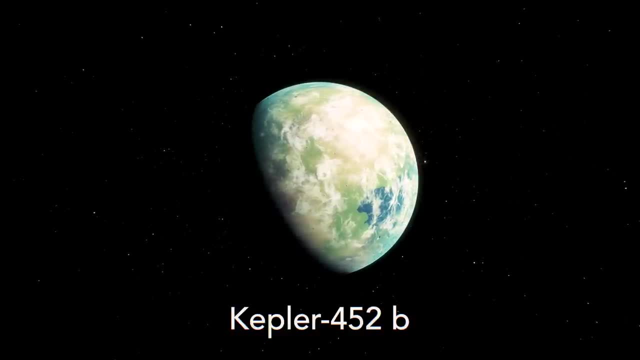 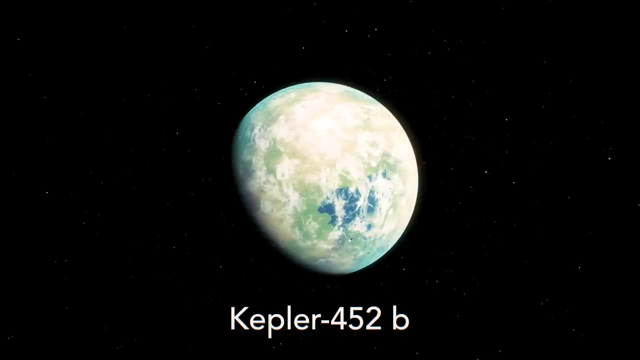 a G2V-type star, Which is a really technical way of saying the same exact type of star as our sun. This means any plants we brought over would be perfectly suited to make use of the light coming in, and any native plant life here has a good chance of being similarly pigmented. 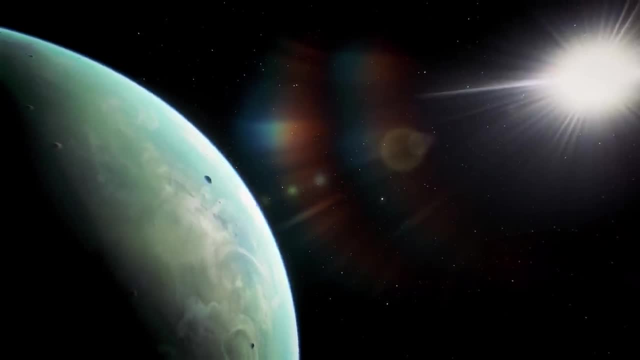 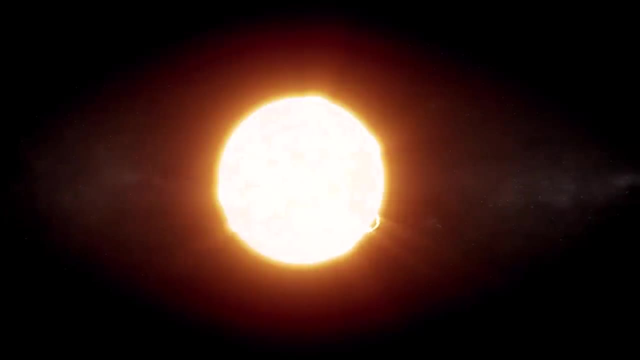 to ours. Though there is one big difference between Kepler-452 and our sun, and that's the star's age Being approximately 6.5 billion years old, 2 billion years older than our sun, the star has already begun to expand. And what is the beginning of the star's age? Well, the star has already begun to expand. And what is the beginning of the star's age? And what is the beginning of the star's age? Well, the star has already begun to expand. 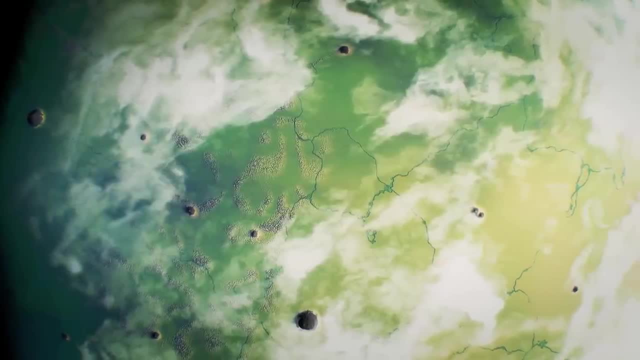 And what is the beginning of the star's age? Well, the star has already begun to expand, So it's not the beginning of its death cycle. While the size of the planet means Kepler-452b would likely be more than able to protect, 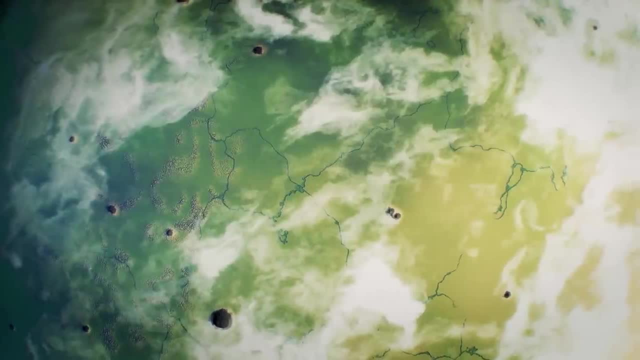 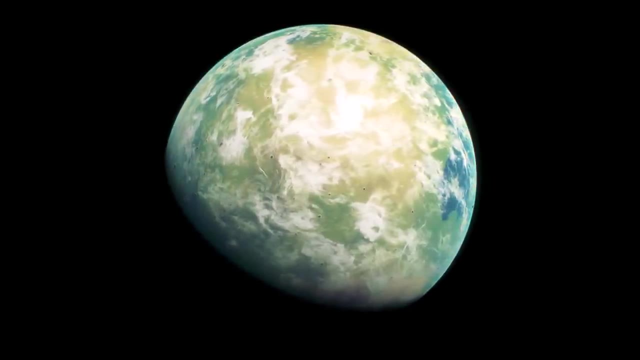 itself against its sun's increasing radiation load for the next couple hundred million years, as a star continues to expand. eventually Kepler-452b will be pushed out of its habitable zone and suffer a runaway greenhouse effect similar to what Venus is experiencing now. 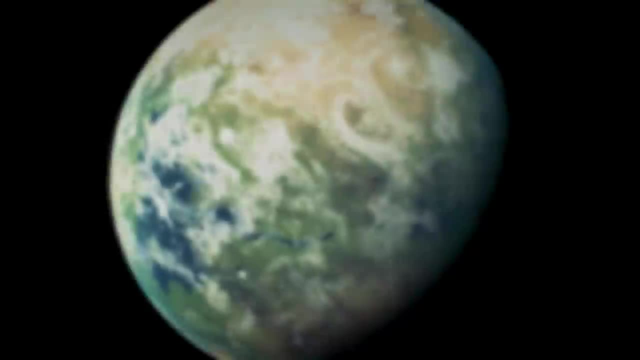 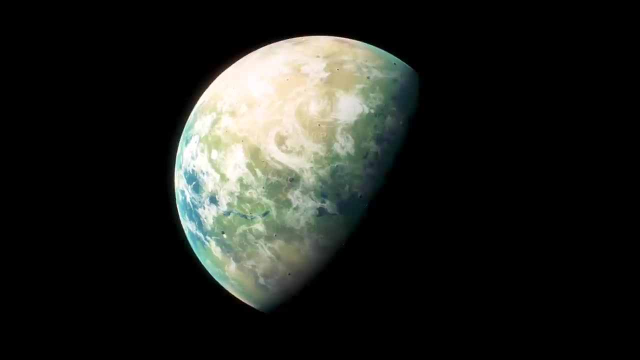 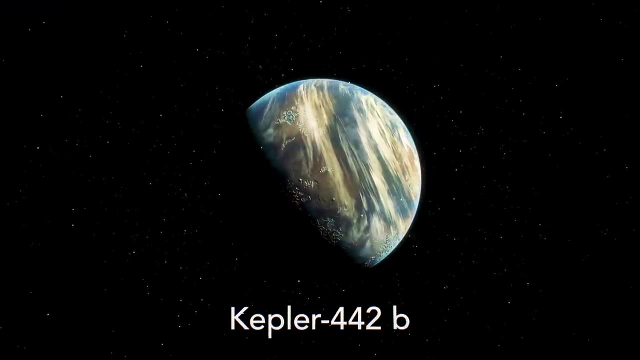 making the surface far too hot to live on. So while in the short term Kepler-452b may be a promising prospect, if we wait until our own sun is dying, 452b will already be long gone. The opposite can be said about Kepler-442b. 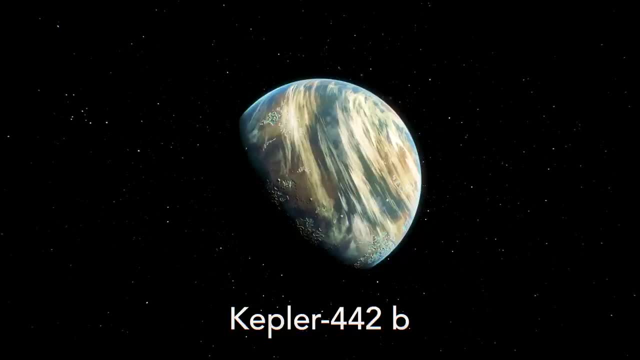 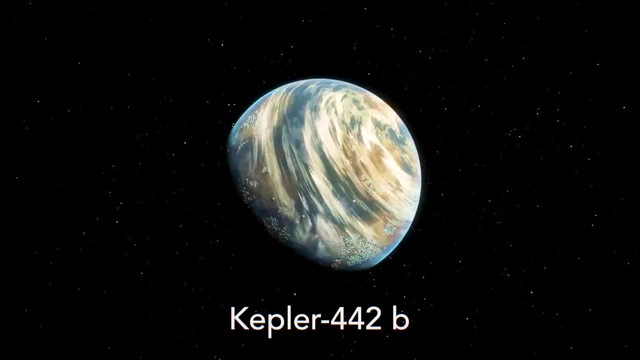 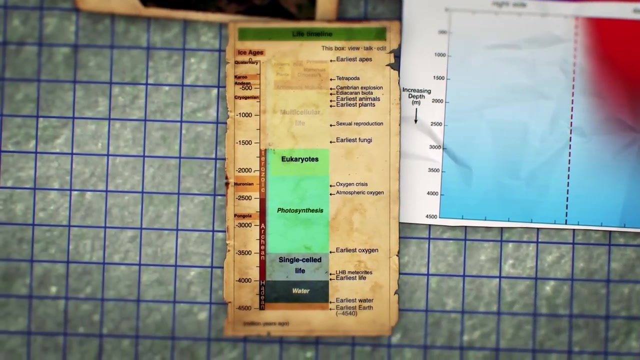 Here we'll find a world only 3 billion years old, a full 1.6 billion years younger than the Earth. If biology here on 442b started and progressed at a similar rate that it did on Earth, that would mean life would just be making its first steps from single cellular to multicellular. 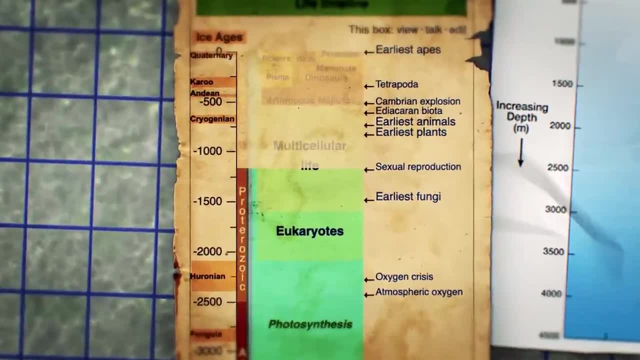 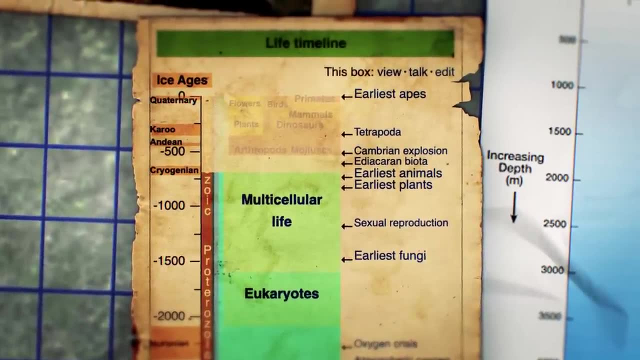 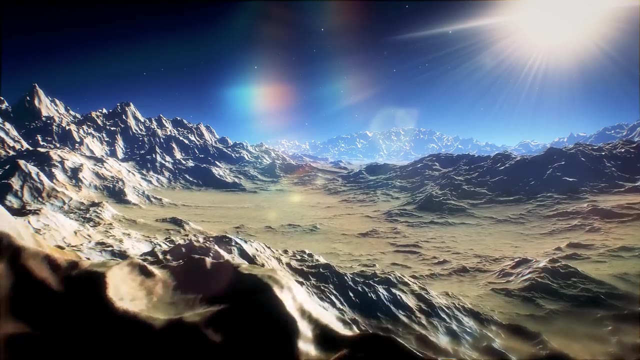 It wouldn't be for another 250 million years that sexual reproduction would come about: 700 million years until plants developed, 800 million years until animals developed and 1.6 billion years before the first potential intelligent life emerged, Which, on the one hand, means we shouldn't expect to find any complex forms of life. 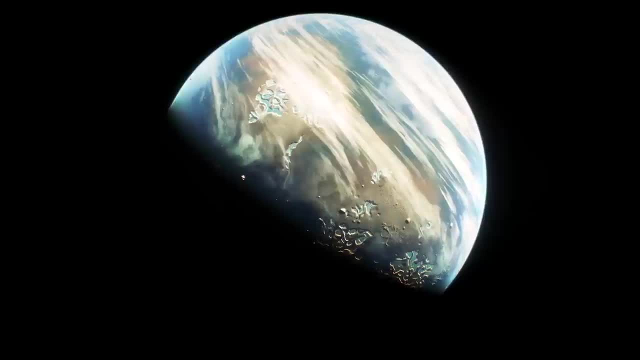 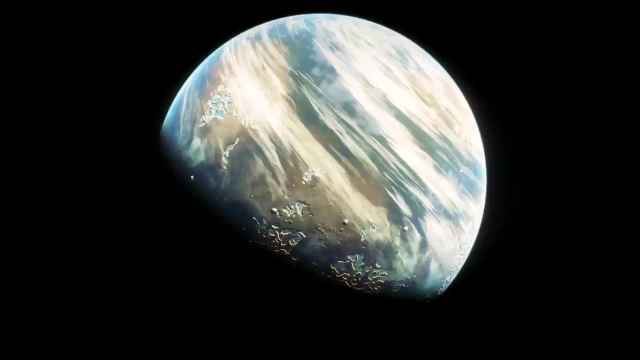 but on the other hand, means the planet is up for the taking. However, we may have reason to believe that life wouldn't necessarily follow the same trajectory here As it did on Earth. You see, at 1.3 times Earth's radius, this not only designates 442b as a super-Earth. 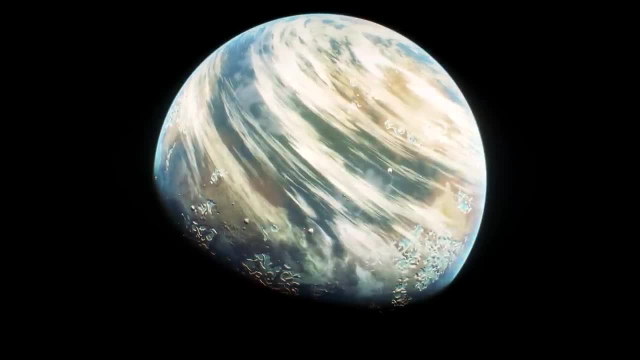 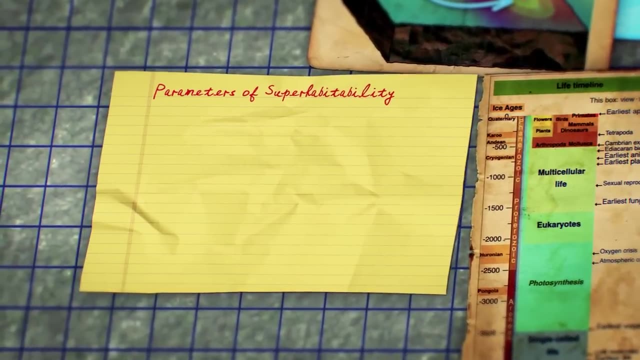 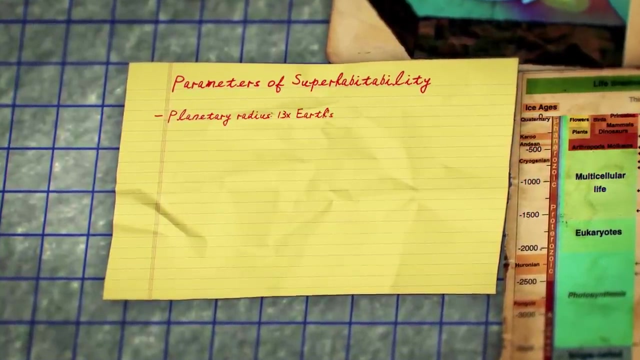 but to some it also qualifies as super-habitable. Now, there are a number of parameters that go into classifying a planet as super-habitable, one of the most important of which I've already mentioned is a planet's size- 442b's- 1.3 times Earth's radius- is thought of as ideal, as this ensures the planet supports. 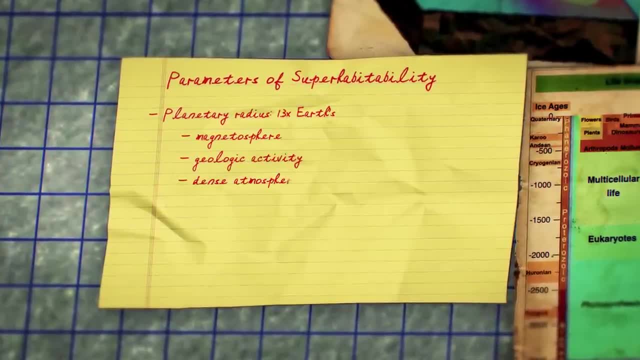 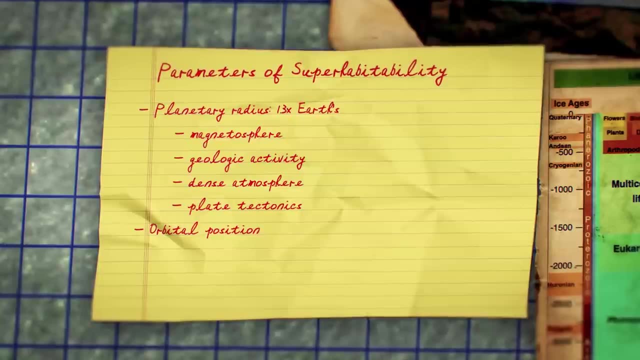 a strong magnetosphere, geologic activity and energy. As you'd probably expect, the planet's orbit also matters, and it just so happens that 442b falls smack-dab in the middle of its star's habitable zone, ensuring the 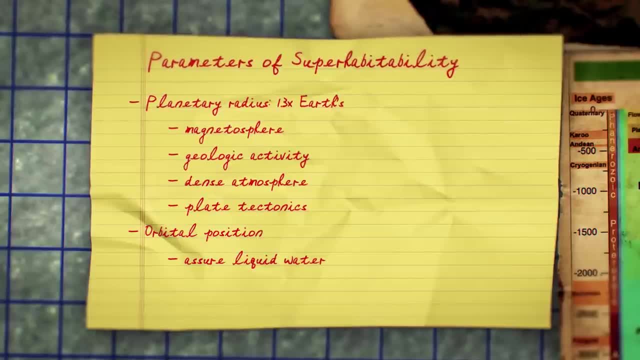 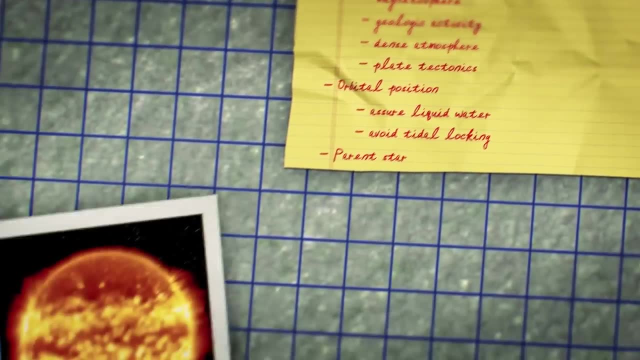 presence of liquid water on its surface, while also keeping far enough away to avoid tidal locking. What a planet orbits also matters, with the ideal type of star not being a G-type star like our own, but rather an M-type or K-type red dwarf like Kepler-4.. 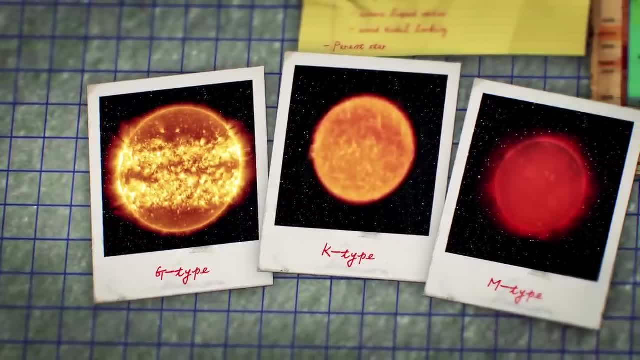 And that's what we're looking for. What a planet orbits also matters, with the ideal type of star not being a G-type star like our own, but rather an M-type or K-type red dwarf like Kepler-4.. That's what we're interested in as well. 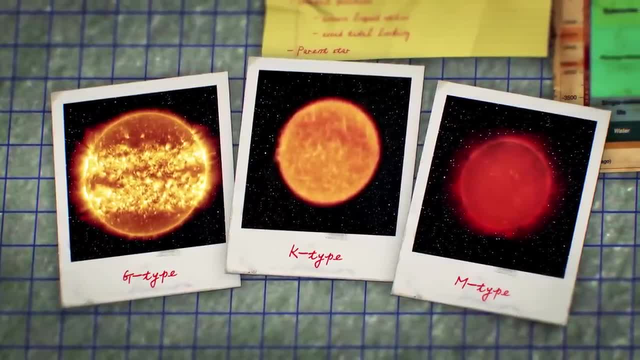 As so many major things at Kepler are about to change, let us talk about some of these. Labrauthor commands here. By this point's has closed the launcher, which Bravo portals power, and to give it some cabalistic background, we really want to talk about another six to seven years. 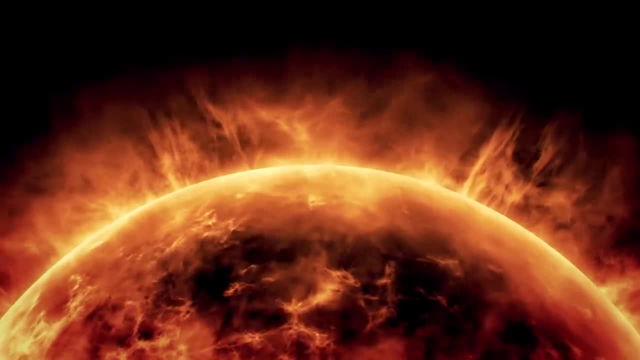 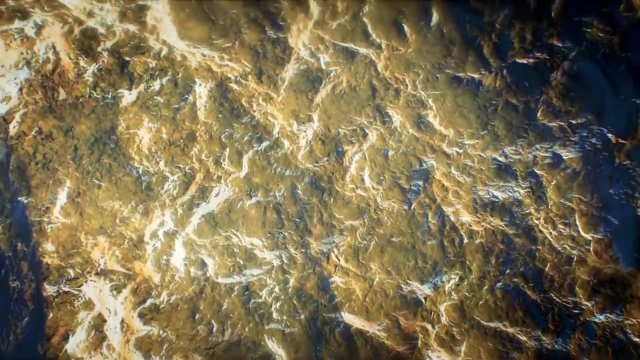 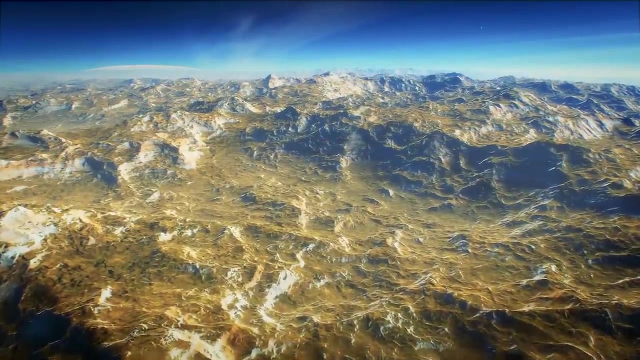 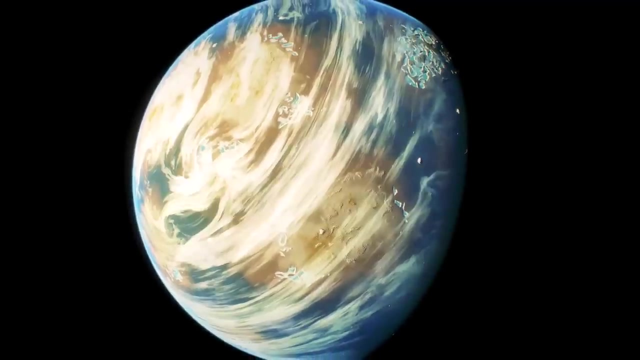 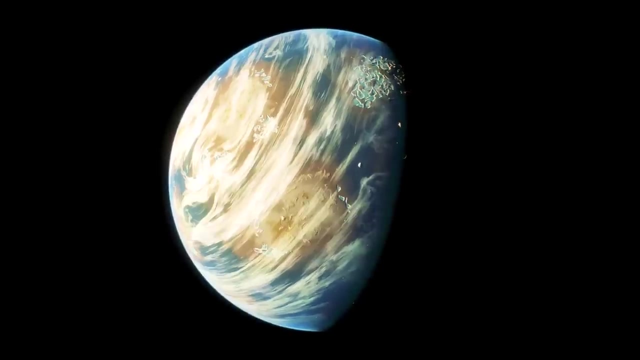 ago in modern history, 4. 4. halten HI 4. 4. 4. 4. at an ESI of 0.84,, though at over 1200 light years away. it's a good thing it has such. 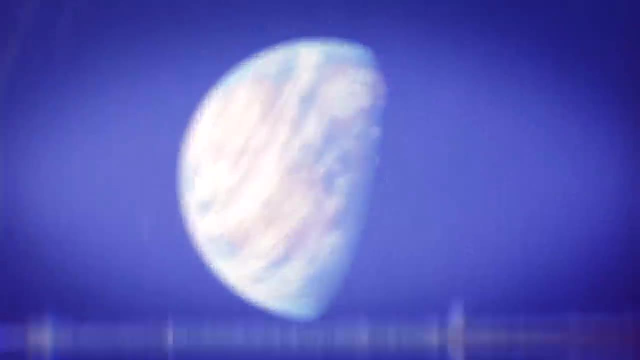 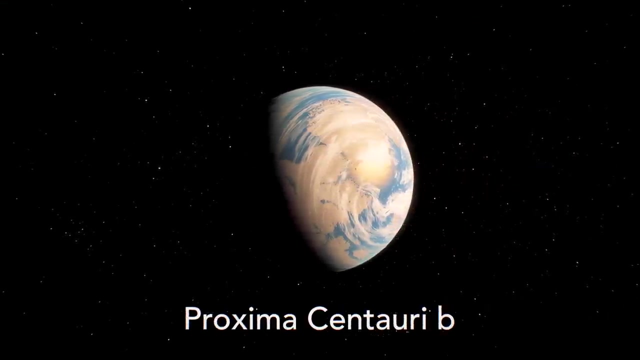 a long lifespan. as it might take us a while to get here. For something a little closer to home, we can move over to our next planet, Proxima Centauri b. If you couldn't tell by the name, Proxima Centauri is very much within our proximity. 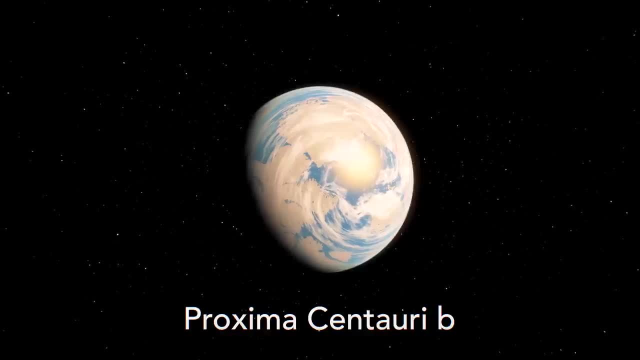 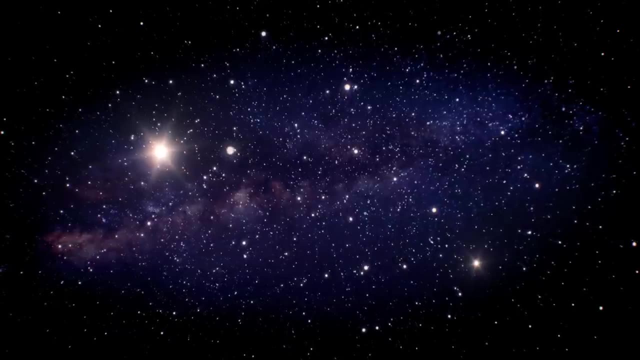 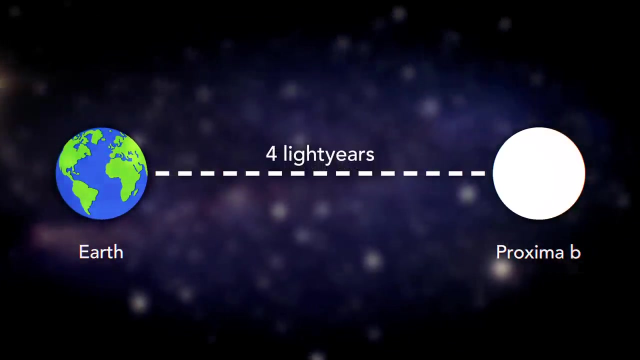 and is actually the closest known star to our solar system and, by extension, this makes the two planets orbiting it the closest known exoplanets to us Traveling at light speed. a trip from the Earth to this system would only take a little over four years, making journeying here more of a possibility than just about anywhere else. 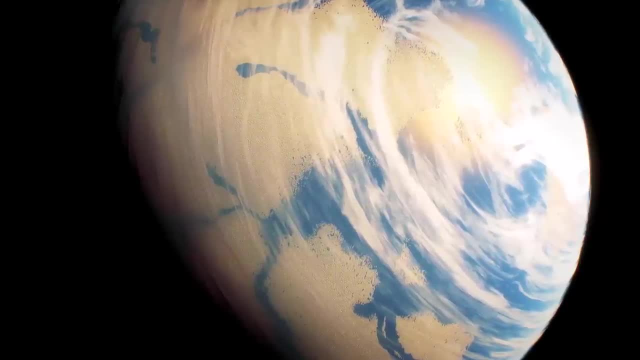 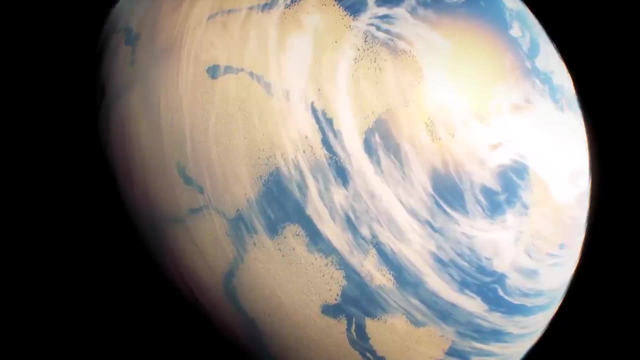 in the galaxy Miraculously. if we did venture here, we'd find a planet roughly the same size as Earth that orbits well within the habitable zone. However, if this all sounds too good to be true, well it might be. You see the parent star Proxima Centauri b. 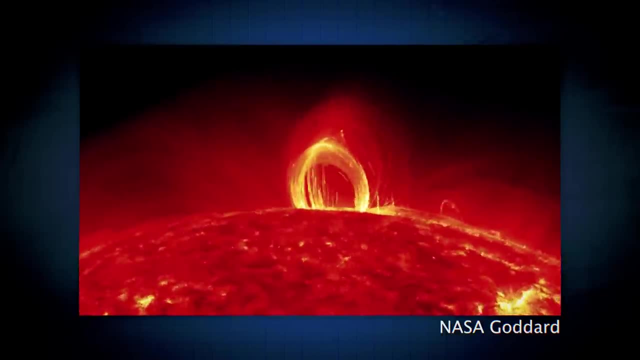 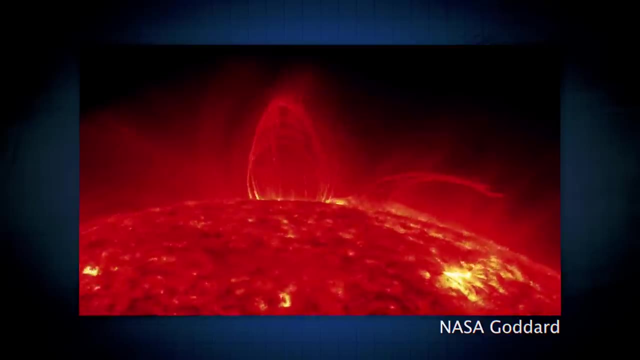 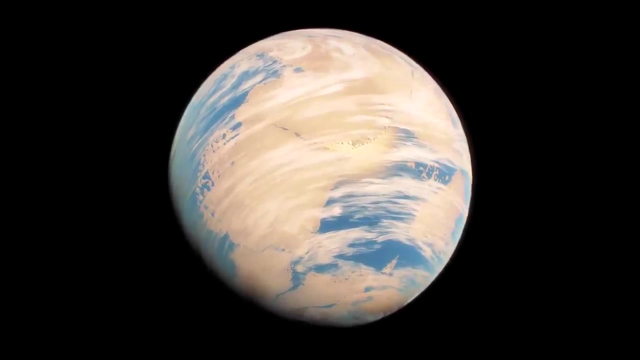 Proxima Centauri is what's called a flare star, capable of randomly emitting huge amounts of radiation, occasionally exposing Proxima b to solar winds over two thousand times stronger than what we experience here on Earth. At levels like this, even a strong magnetosphere may not be enough to protect the planet's. 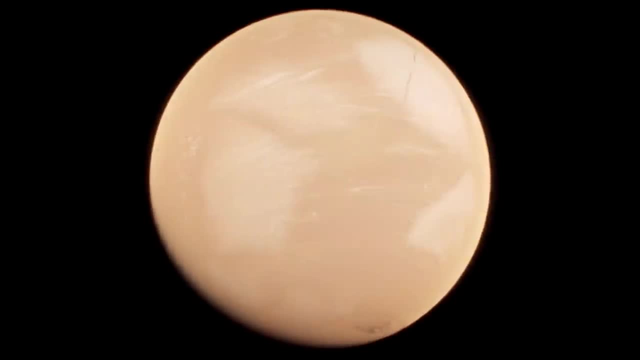 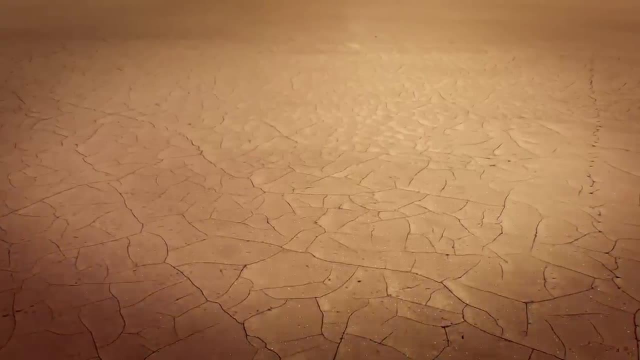 atmosphere from vaporizing away, potentially leaving the surface exposed to the harsh environment of space. While life is still theoretically possible here, it would be relegated to the planet's subsurface. It would offer just enough protection from the sporadic solar flares to harbor simple. 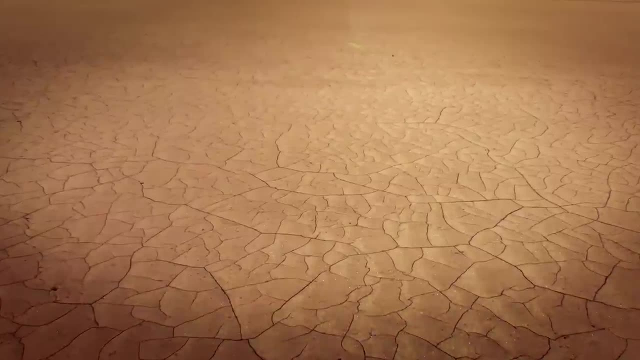 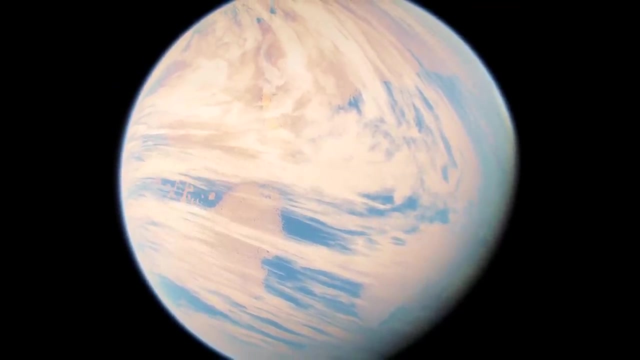 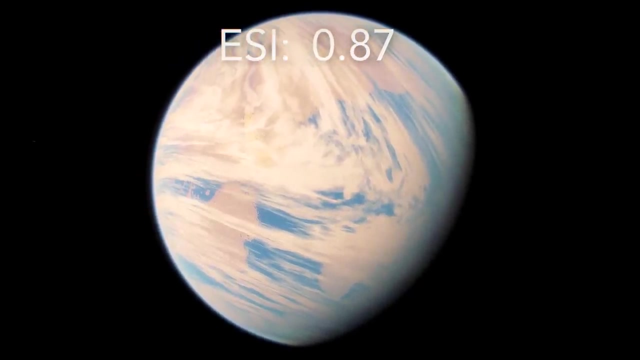 life forms. Whether or not life could first emerge in an environment like this is another story. Overall, despite these challenges, the surface level similarities Proxima b shares with Earth earns the planet an ESI of 0.87,, though this has a high likelihood of changing in the near. 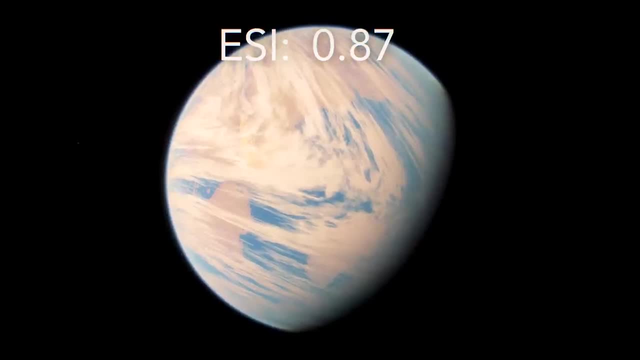 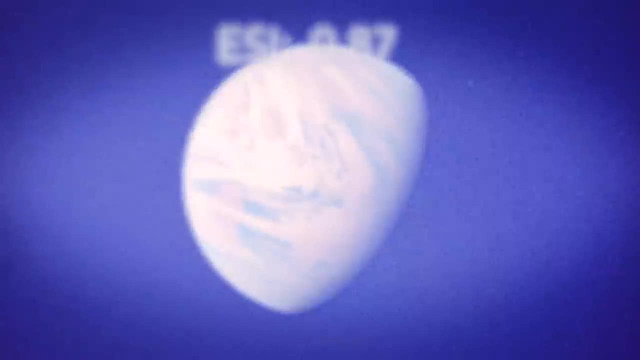 future as, being so close to Earth, we may be able to observe the planet through the next generation of advanced telescopes and get answers to some of the most pressing questions If we want a planet with a bit more quiet of a host star, but still pretty close to us. 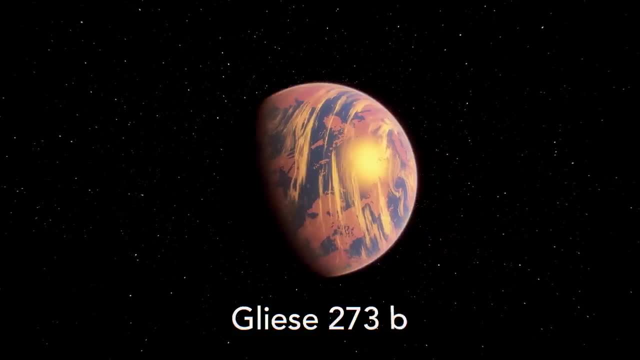 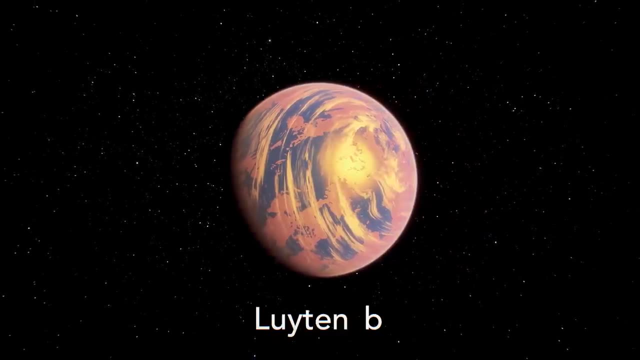 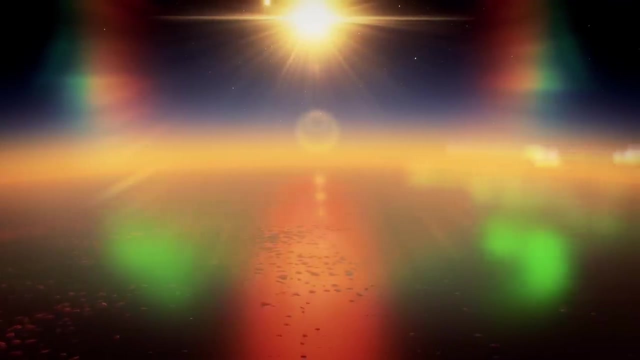 we can look no further than Gliese 273 b, otherwise known as Leighton b, At a distance of only 12 light years away. 273 b remains in our general neighborhood while managing to orbit what appears to be a very quiet star With a luminosity of only 0.88% to that of the sun, in order to occupy the habitable zone. 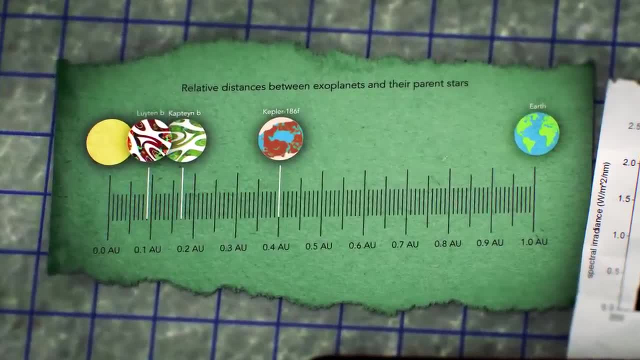 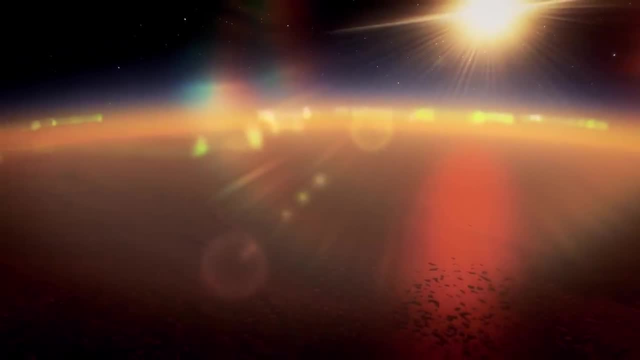 Leighton b must orbit extremely close to Earth At only 0.09 AU, likely tidally locking the planet. Though with such a peaceful star, Leighton b is likely able to have a substantial atmosphere, greatly improving the planet's potential habitability to everywhere not directly under. 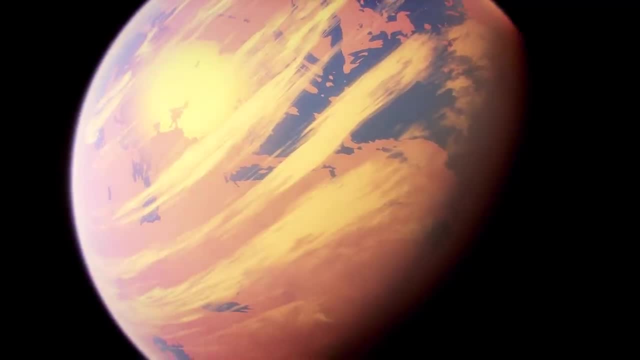 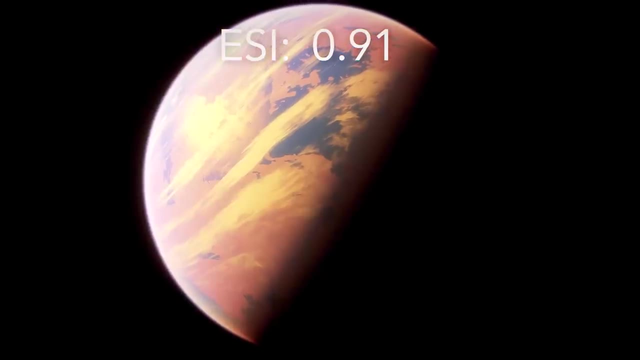 the focus or directly opposite. All of this combined results in a planet with an ESI of 0.91, an exceptionally high score, with only three other confirmed exoplanets ranking higher. Next we're traveling to Teegarden's Stone. 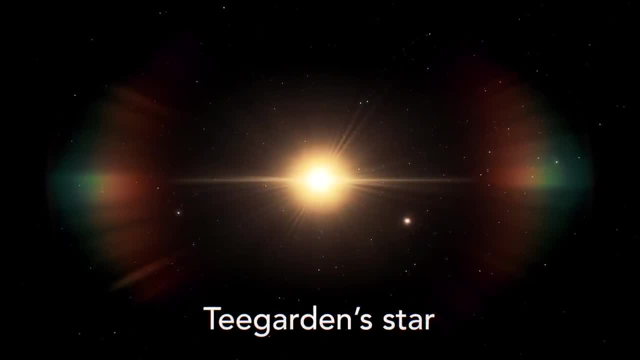 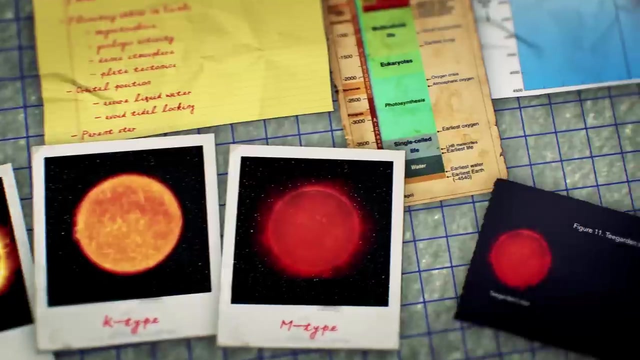 Very similar to Leighton. here we'll find a small red dwarf only 12 light years away, with a low level of activity. What makes Teegarden so special is that it hosts not one, but two rocky planets within its habitable zone: Teegarden b and Teegarden c. 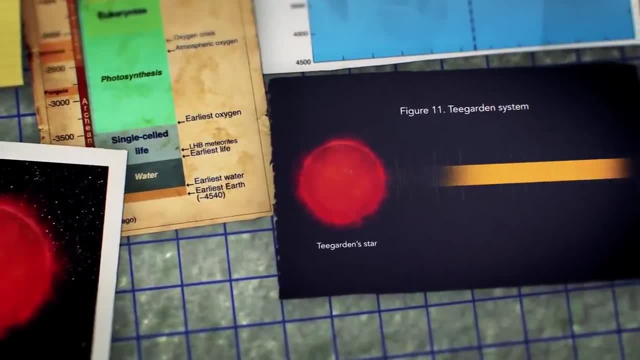 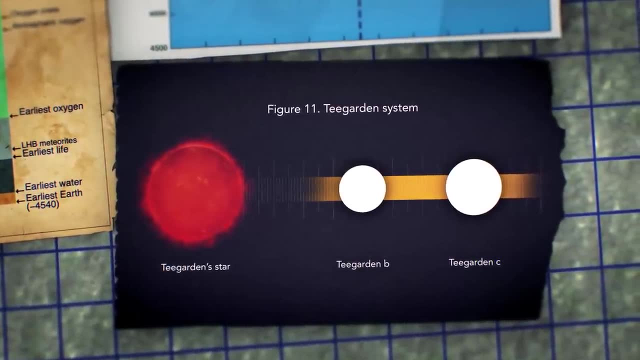 In order for both planets to occupy Teegarden's narrow habitable zone, they need to be relatively far apart from one another, putting b far on the warmer side of the zone and c further on the colder side. Here we'll find a good example of why a planet's earthlikeness doesn't always equate. 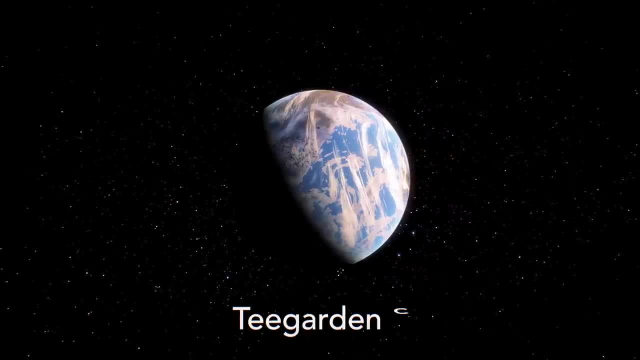 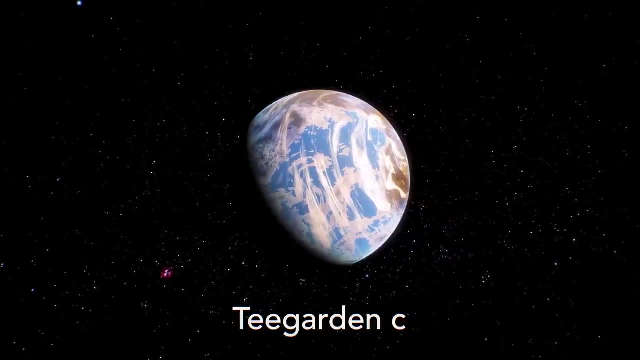 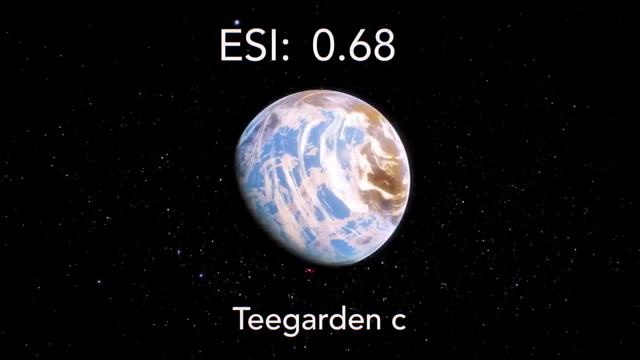 to habitability. Being on the cold side, Teegarden c's larger-than-earth size would likely help the planet trap more heat and support bodies of water, making it overall more habitable, while simultaneously less earthlike In total, earning the planet an ESI of only 0.68, despite its good chances for maintaining. 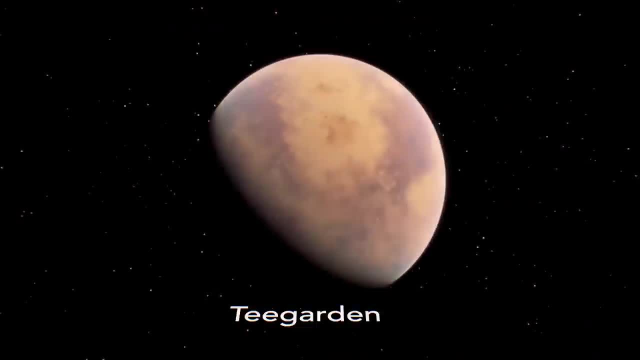 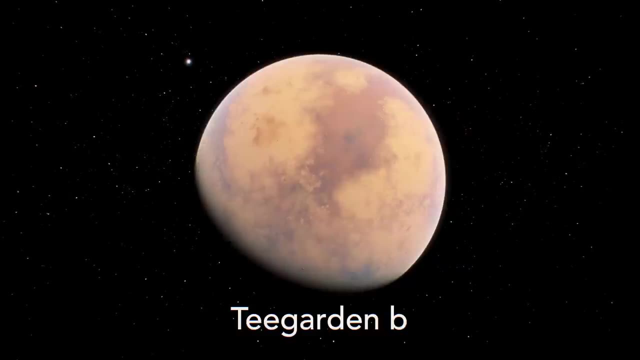 bodies of water on its surface. Meanwhile, Teegarden b strays critically close to the inner ring of its habitability. Teegarden c is a habitable zone, running the risk of excessive greenhouse heating and diminishing its chances of hosting a habitable environment. 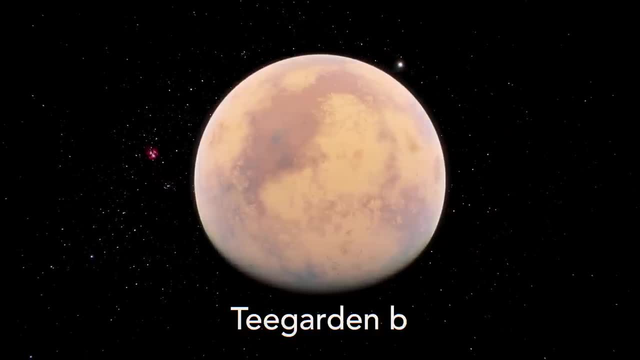 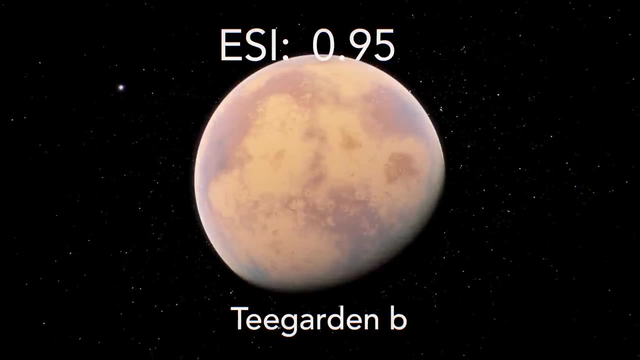 Despite this, with a more earth-like mass of 1.05,, b earns an ESI of 0.95,, the highest of any exoplanet discovered to date. Normally this would be enough to earn the status of Earth 2.0, but well, I'm not convinced. 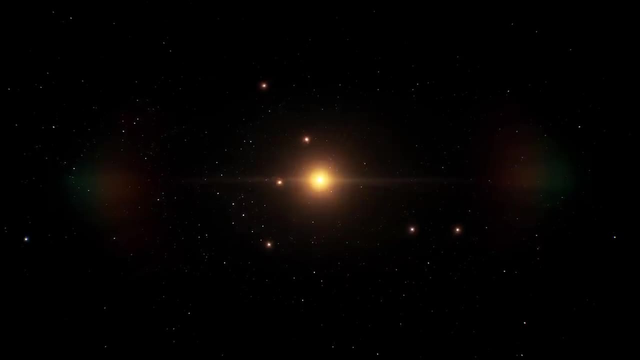 This just doesn't feel like the best we can do. So, finally, it's time to talk about the Trappist-1 system, or what can only be described as the most remarkable discovery in exoplanets to date, with not one, not two, not even three. 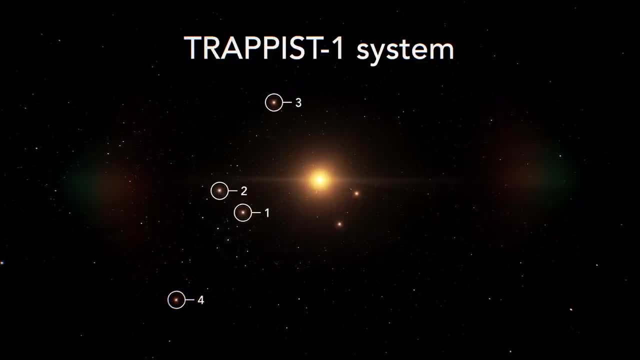 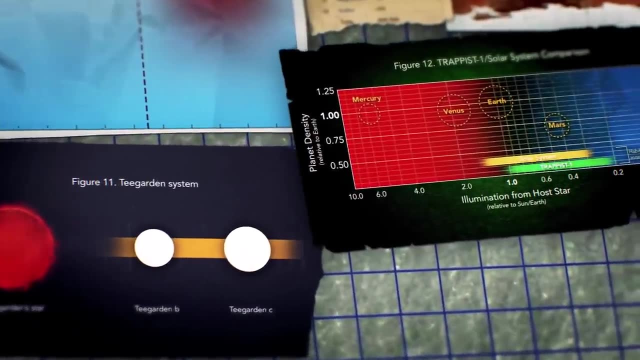 but four planets orbiting within its habitable zone, out of a total of seven. Comparing the position of the planets of the Trappist-1 system to those of our solar system, we'll see that while Trappist-1, b and c orbit too close- even closer than Venus- sits Trappist-1. 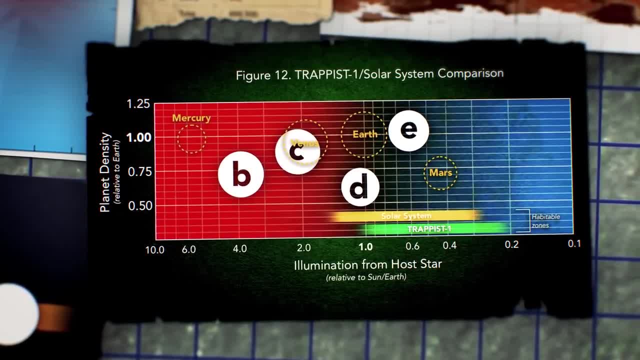 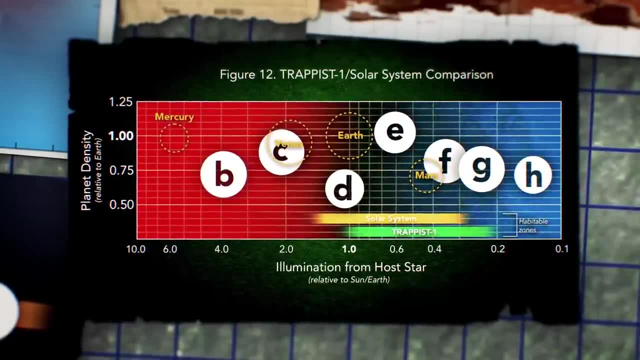 d sits just ahead of Earth, e comfortably between Earth and Mars, and f and g falling slightly behind, It's still within their star's habitable zone. with h lurking too far back, Starting with Trappist-1 g, we'll find the coldest of the habitable Trappist planets. 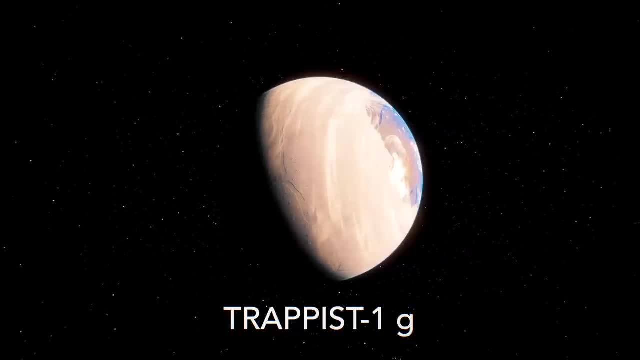 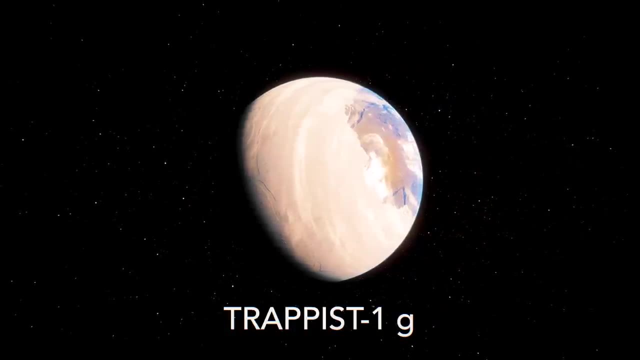 Analysis of the planet found it had a density 76% that of Earth, a strong indicator that a large amount of the material constituting the planet comes in the form of water. Being on the colder side of things, it's likely that most of this water comes in the form. 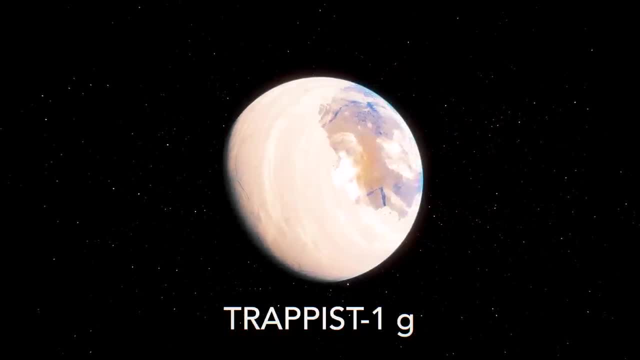 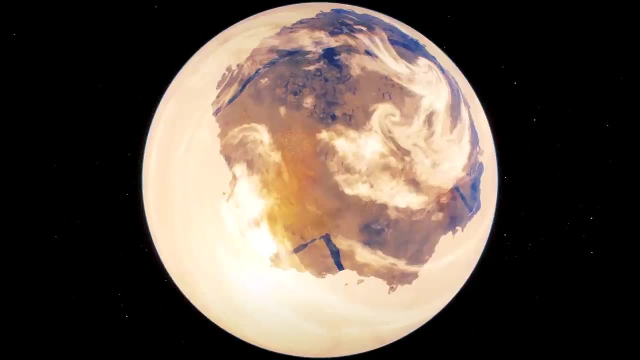 of colossal ice sheets covering the vast majority of the planet. However, the Earth, Mars and the Earth itself are tightly locked, meaning around the focus. these ice sheets could thin out and even entirely thaw, opening a small muddy area at the center. 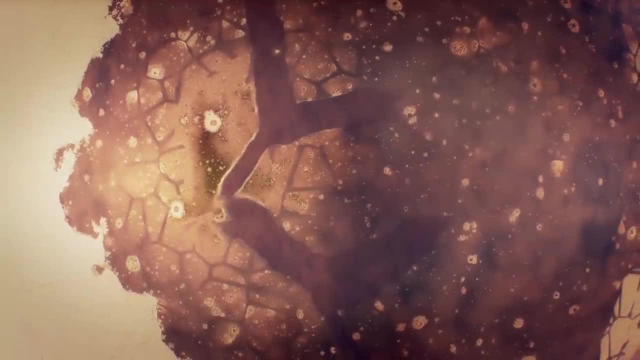 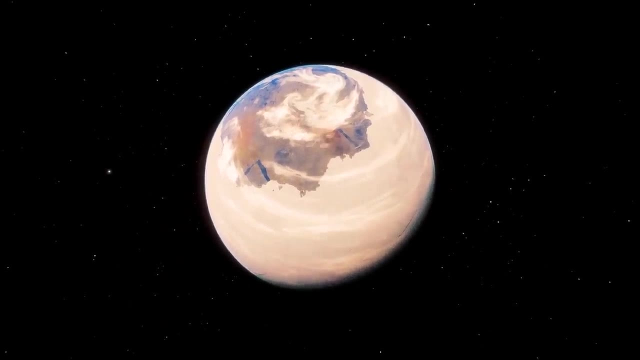 of the planet where meltwaters likely run through to possibly feed into lakes. Overall, this gives the planet the appearance of a hatching egg or an eyeball For an example of what a similar, if slightly warmer, planet would look like. we can move. 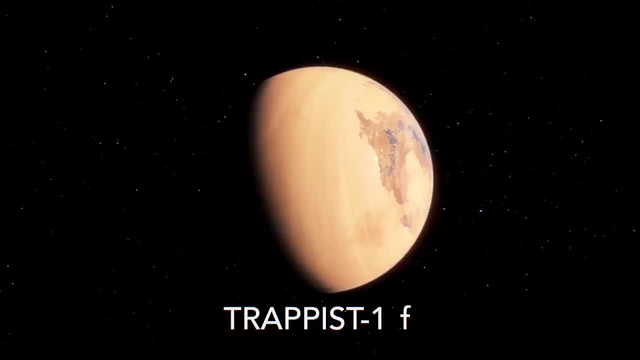 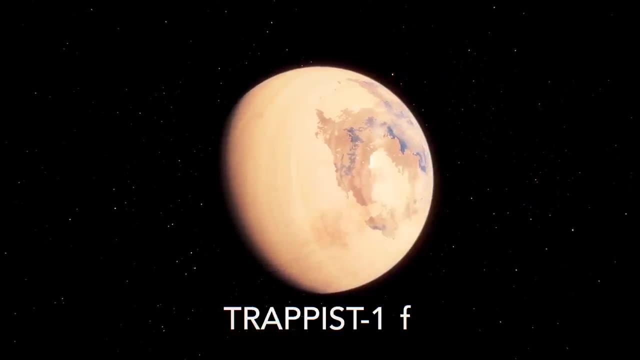 on over to Trappist-1 f, The next furthest planet in the Trappist lineup. Here we'll find a similar eyeball planet only being closer to the parent star. the encompassing ice sheets have been pushed much further back, opening a wider focus crater. 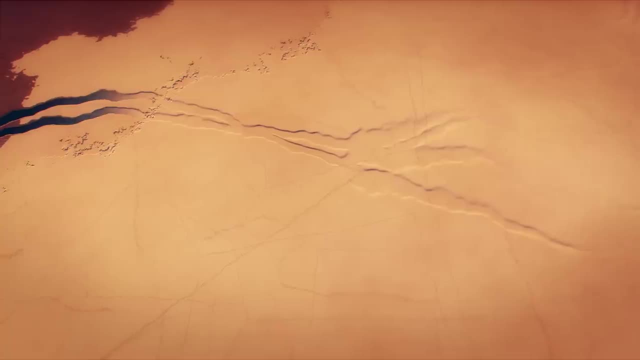 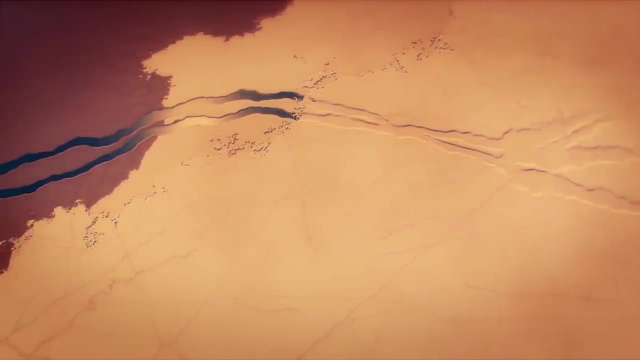 for more substantial water bodies to fill With an almost identical radius to Earth, but only 68% its mass. this is expected to be another water-rich world, with calculations proposing the composition of the planet to be up to 20% water. 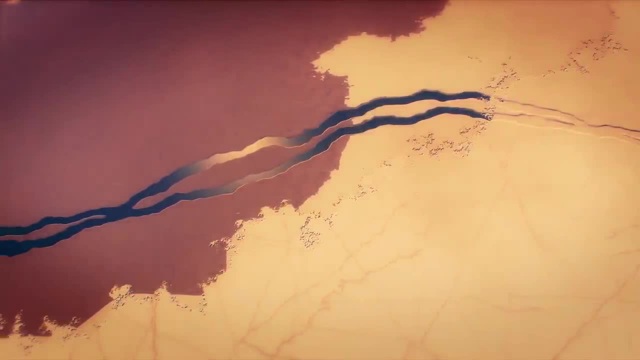 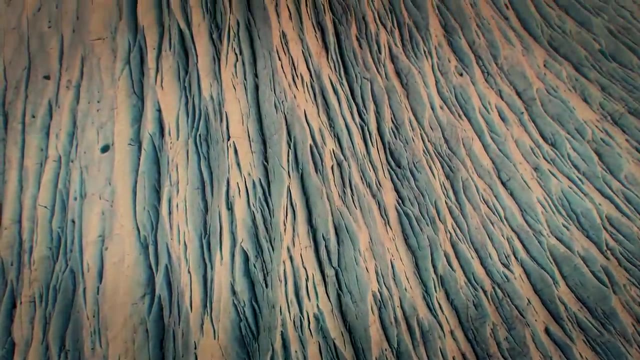 For comparison, Trappist-1 f only makes up 0.02% of the Earth's mass, meaning. here, on 1 f, this great quantity of water would build ice sheets tens, even hundreds of miles deep. This makes me think that not only could sizeable lakes occupy the focus, but rather a single. 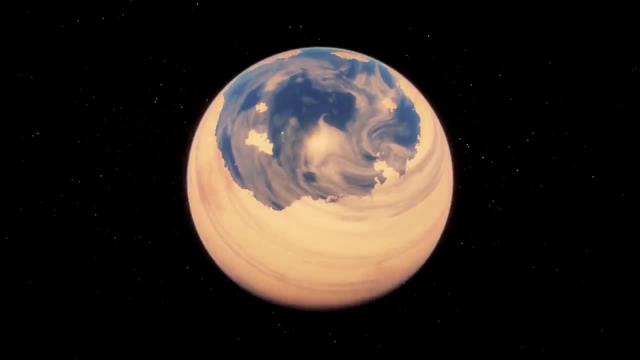 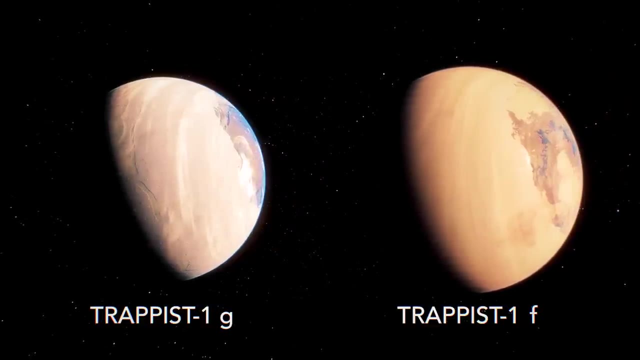 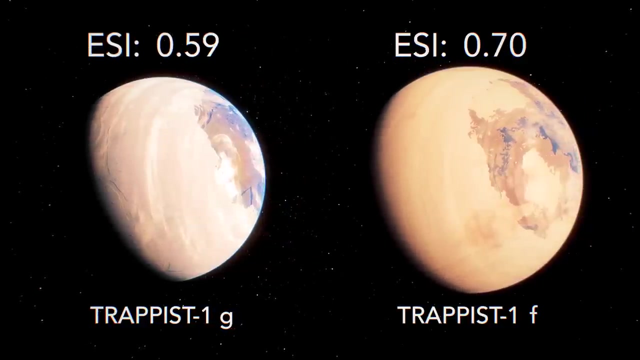 huge ocean, nearly as deep as the ice surrounding it, making the planet essentially one big fishbowl. For their differing sizes and compositions, Trappist-1 f and g earn ESIs of only 0.70, and 0.59, respectively, meaning we can still do better. 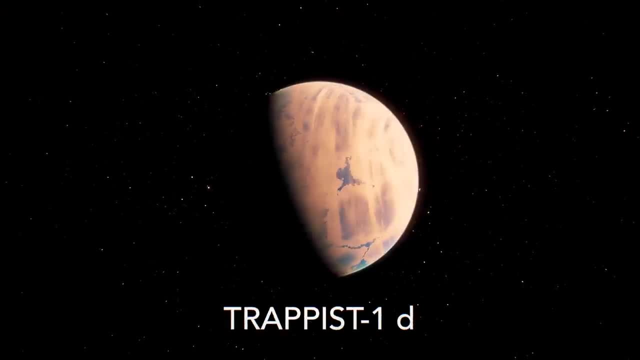 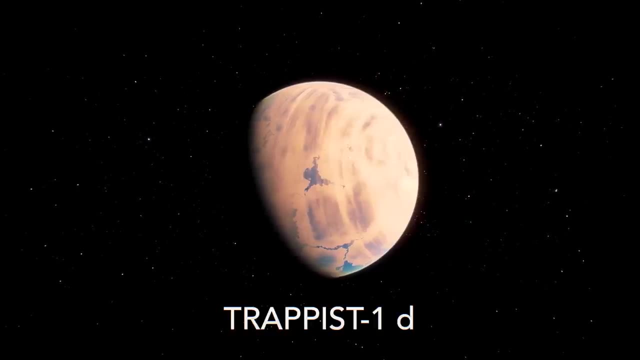 So now we're moving on to Trappist-1 d, Again with a lower density than Earth. d is also expected to harbor large amounts of water, though this may in fact be mostly in the gaseous form rather than liquid encasing the planet. 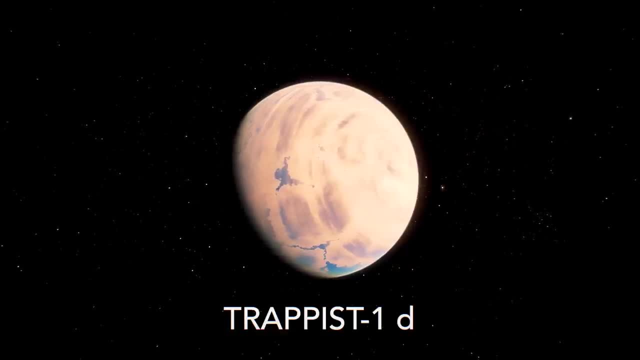 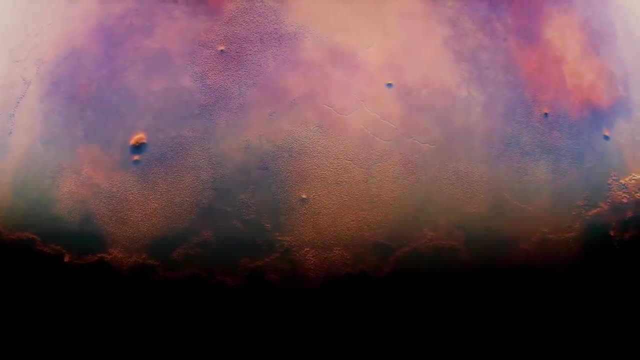 in a thick and swampy water vapor atmosphere more akin to Venus. This, however, opens up an interesting possibility where the excessive heat of the planet's focus makes the day side utterly uninhabitable, But it generates a far more temperate climate across the night side of the planet. 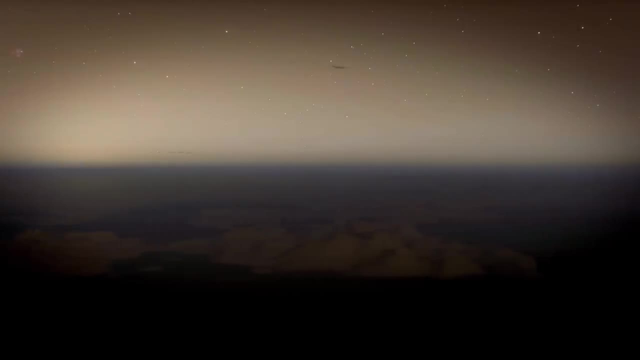 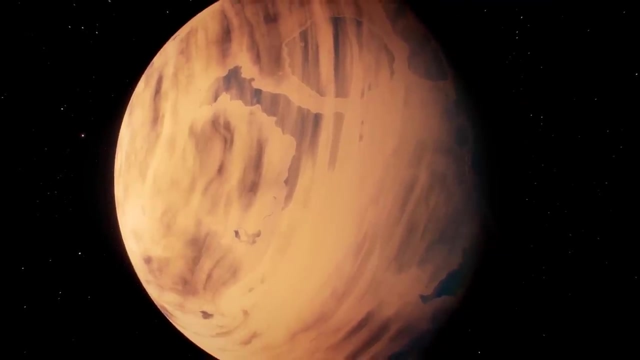 Here lakes or even oceans of water could be sitting in absolute darkness, providing a refuge for life steeped in fog and forever under the stars. Overall simulations of conditions on the planet are split between an Earth-like and a more Venus-like world, but either way, the possibility for life is real and the planet 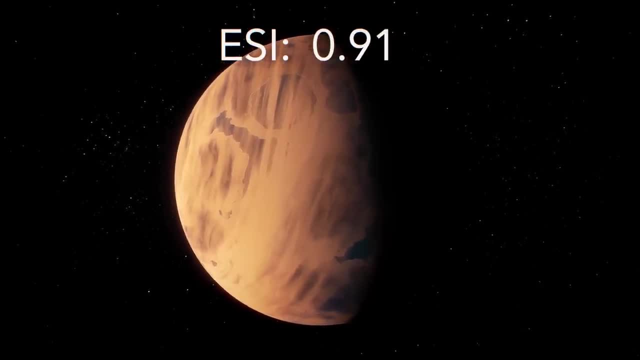 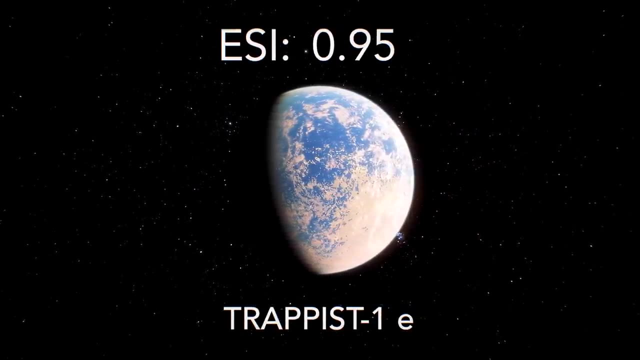 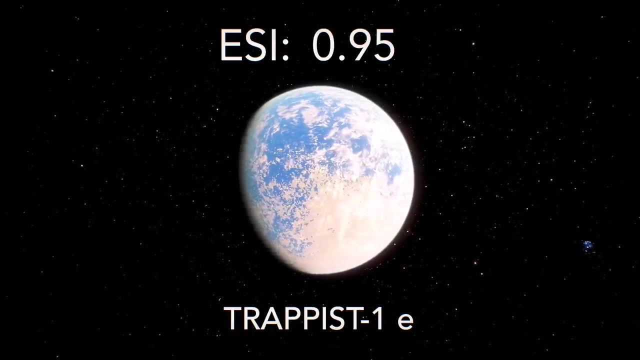 earns a total ESI score of 0.91.. Finally, this leaves Trappist-1 d With an ESI score of 0.95,. together with Teegarden b, this represents the most Earth-like exoplanet discovered and confirmed to date. 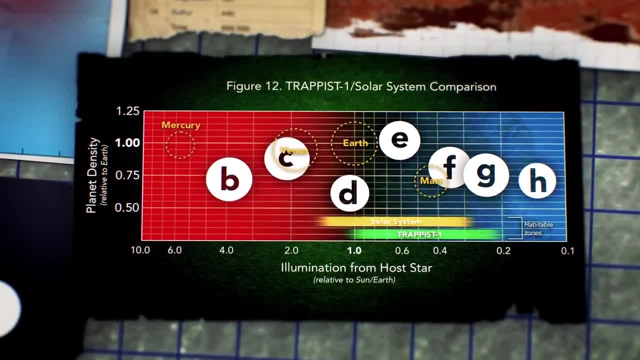 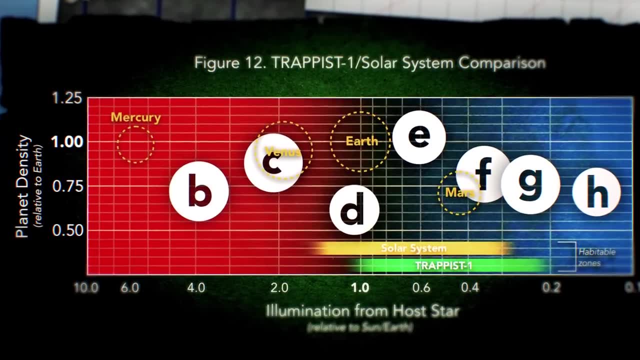 We can see this reflected in where e is located back on our chart, being situated slightly on the warm side of the habitability zone, just like us, and with a size and density nearly identical to the Earth. With a greater density, the planet is less likely to contain the copious amounts of water.